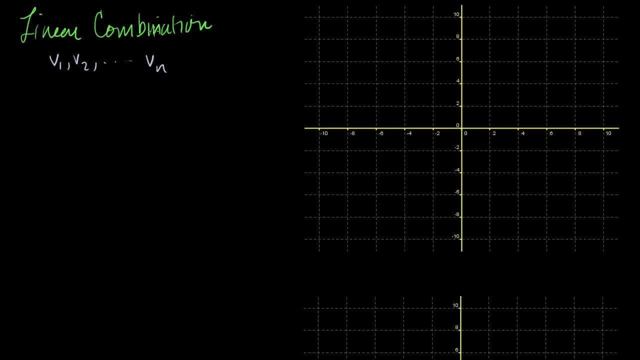 goes all the way to vn And they're all in. you know it can be an r2 or rn. Let's say that they're all in rn. They're in some dimension of real space, I guess we could call it. 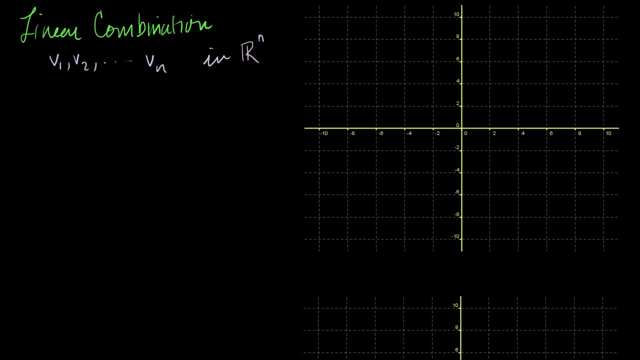 But the idea is fairly simple. A linear combination of these vectors means you just add up the vectors. It's some combination of a sum of the vectors, so v1 plus v2 plus all the way to vn. But you scale them by arbitrary constants. 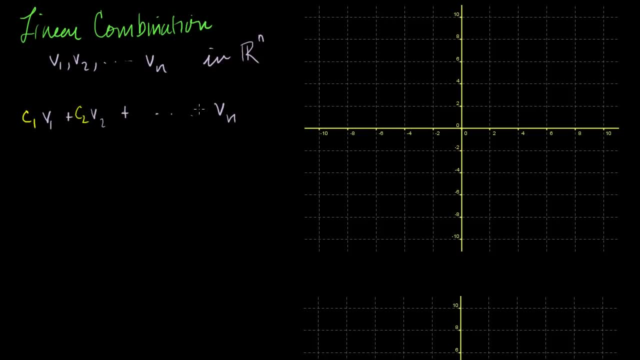 So you scale them by c1.. c1, c2, all the way to cn, where everything from c1 to cn are all a member of the real numbers. That's all a linear combination is, And let me show you a concrete example of linear. 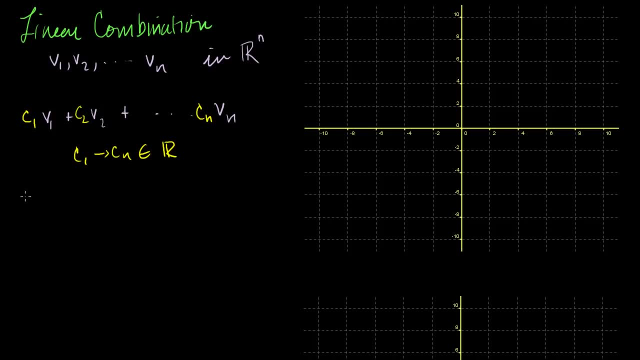 combinations. Let me make the vector, let me define the vector a to be equal to. and these are all bolded. these purple v's are all bolded just because those are vectors, But sometimes it's kind of onerous to keep. 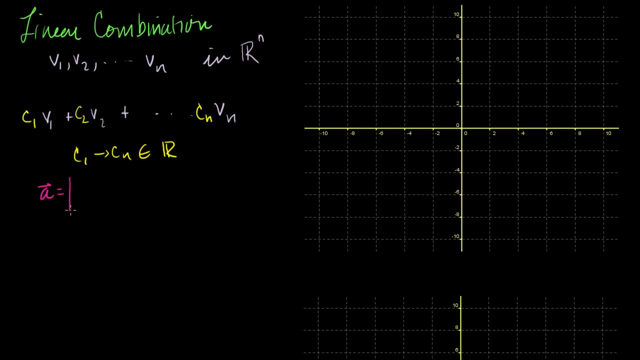 bolding things. So let's just say: I define the vector a to be equal to, you know, 1, 2, and I define the vector b to be equal to 0, 3.. What is a linear combination of a and b? 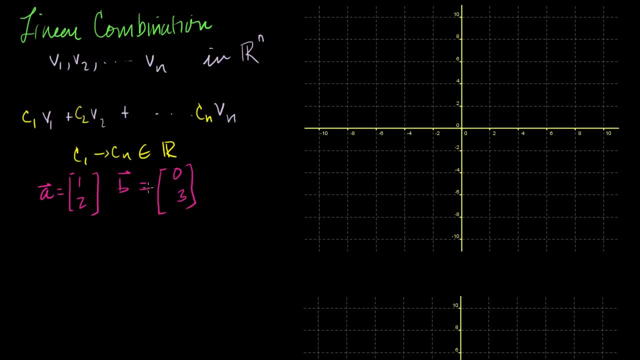 Well, I could. just, it gives you any constant times a plus any constant times b, So it could be 0 times a plus. well, it could be 0 times a plus 0 times b, which, of course, would be what. 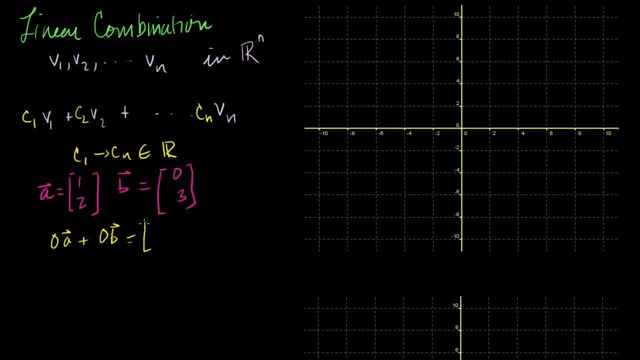 That would be 0 times a would be 0, 0, and 0, 0,. that would be the 0 vector. but this is a completely valid linear combination and we can denote the 0 vector by just a big. 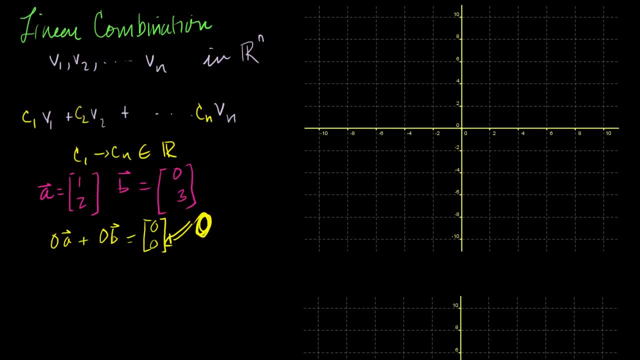 bold 0 like that We could also. this is almost I could do- 3 times a. I'm just picking these random, these numbers at random: 3 times a plus let me do a negative number just for fun. So let's do plus minus 2 times b. 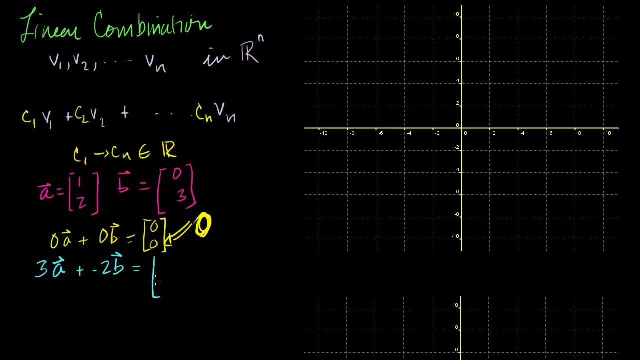 What is that equal to? Well, let's figure it out. Let me write it out: It's minus. it's 3 minus 2 times 0,, so minus 0, and this 3 times 2 is 6,, 6 minus 2 times 3,, so minus 6.. 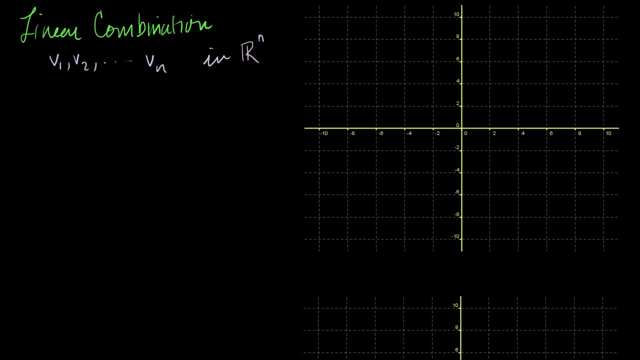 But the idea is fairly simple. A linear combination of these vectors means you just add up the vectors. It's some combination of a sum of the vectors, so v1 plus v2 plus all the way to vn. But you scale them by arbitrary constants. 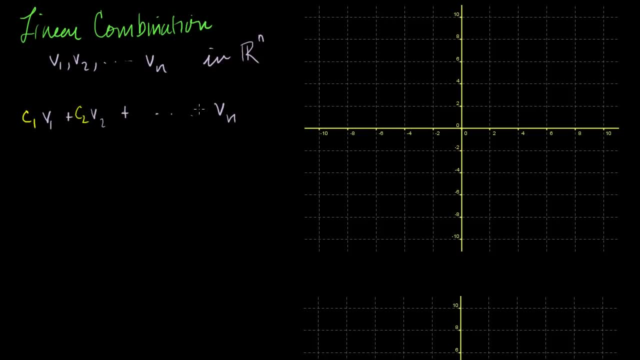 So you scale them by c1.. c1, c2, all the way to cn, where everything from c1 to cn are all a member of the real numbers. That's all a linear combination is, And let me show you a concrete example of linear. 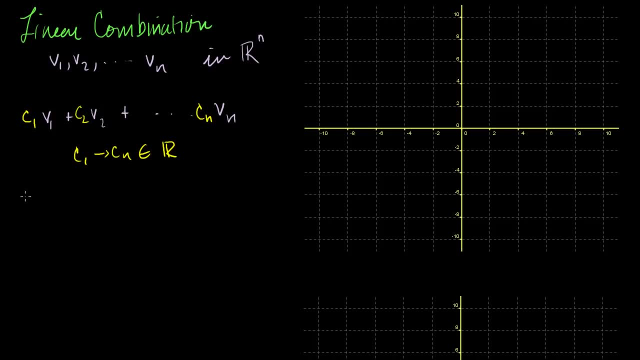 combinations. Let me make the vector, let me define the vector a to be equal to. and these are all bolded. these purple v's are all bolded just because those are vectors, But sometimes it's kind of onerous to keep. 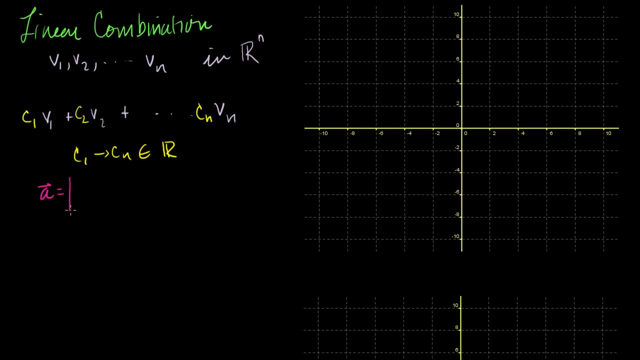 bolding things. So let's just say: I define the vector a to be equal to, you know, 1, 2, and I define the vector b to be equal to 0, 3.. What is a linear combination of a and b? 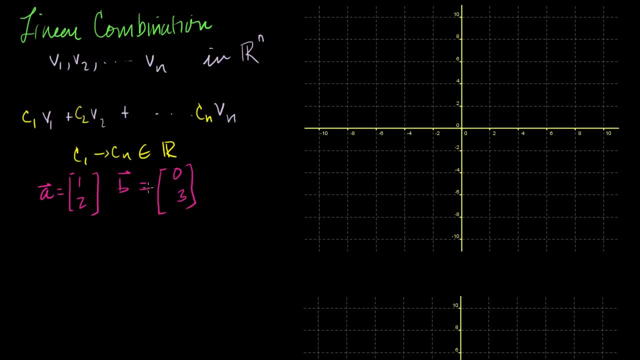 Well, I could. just, it gives you any constant times a plus any constant times b, So it could be 0 times a plus. well, it could be 0 times a plus 0 times b, which, of course, would be what. 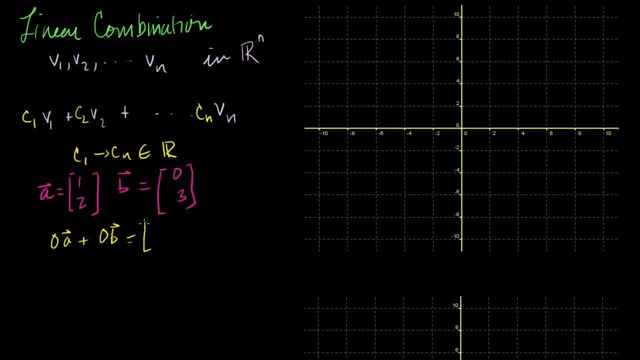 That would be 0 times a would be 0, 0, and 0, 0,. that would be the 0 vector. but this is a completely valid linear combination and we can denote the 0 vector by just a big. 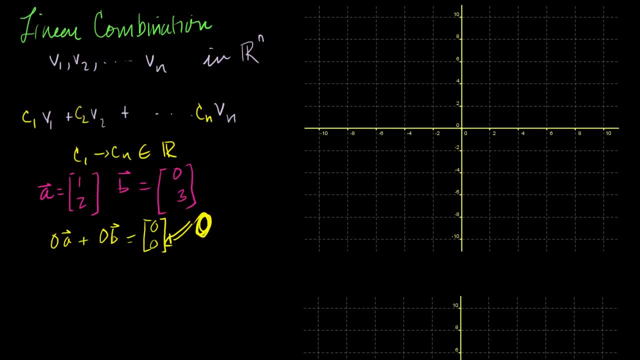 bold 0 like that We could also. this is almost I could do- 3 times a. I'm just picking these random, these numbers at random: 3 times a plus let me do a negative number just for fun. So let's do plus minus 2 times b. 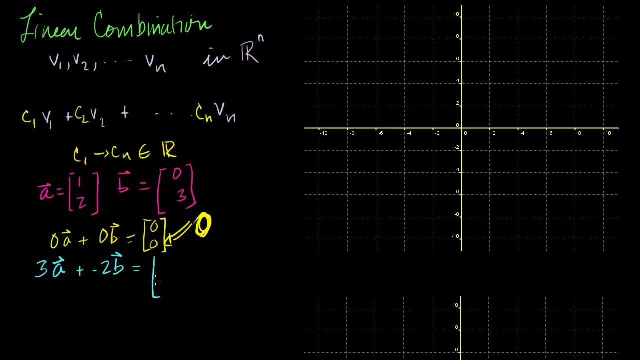 What is that equal to? Well, let's figure it out. Let me write it out: It's minus. it's 3 minus 2 times 0,, so minus 0, and this 3 times 2 is 6,, 6 minus 2 times 3,, so minus 6.. 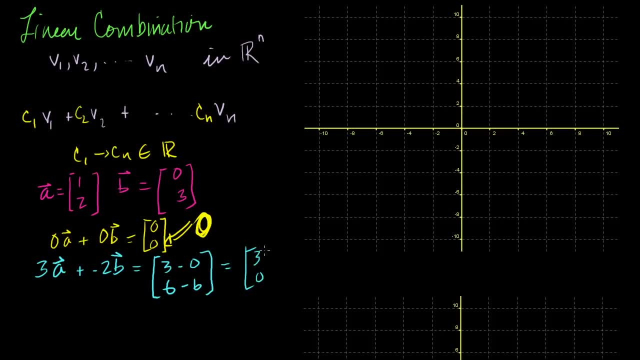 So it's the vector 3,, 0.. This is a linear combination of a and b. I could keep putting in a bunch of random real numbers here and here and I'll just get a bunch of different linear combinations of my vectors a and b. 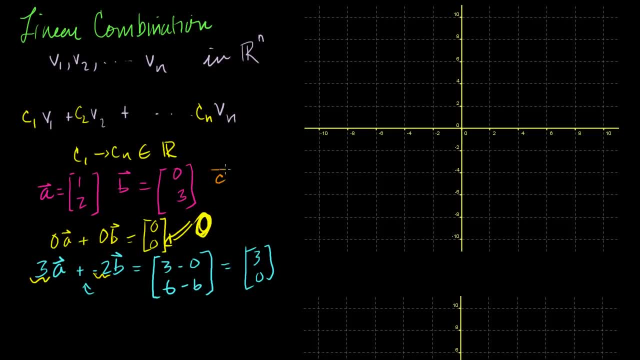 If I had a third vector here, if I had vector c- and maybe that was just 7, 2, then I could add that to the mix and I could throw in plus 8 times vector c. These are all just linear combinations. 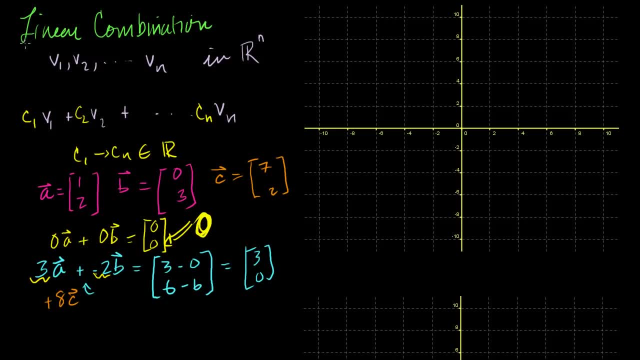 Now why do we just call them combinations? Why do we have to add that little linear prefix there? Because we're just scaling them up. We're not multiplying the vectors times each other. We haven't even defined what it means. It means to multiply a vector and there's actually several. 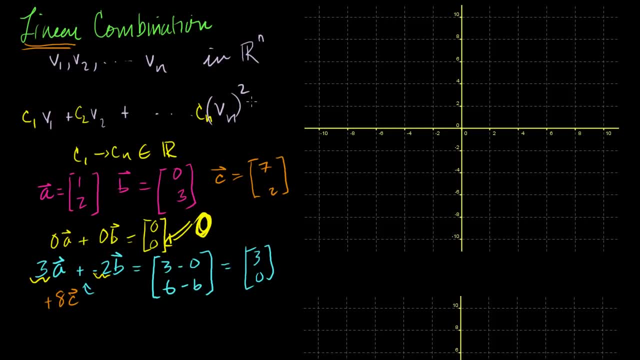 ways to do it, But we can't square a vector, and we haven't even defined what this means yet. but this would all of a sudden make it nonlinear in some form. So all we're doing is we're adding the vectors and we're 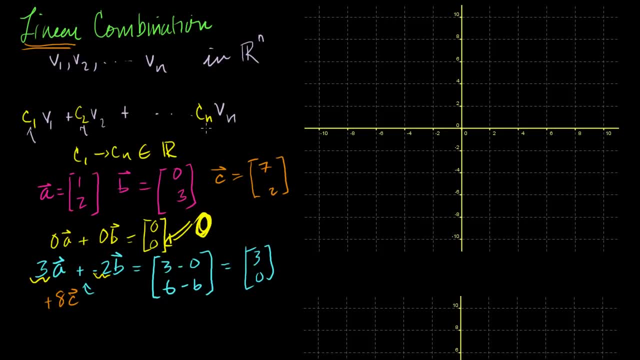 just scaling them up by some scaling factor. So that's why it's called a linear combination. Now you might say: hey Sal, why are you even introducing this idea of a linear combination? Because I want to introduce the idea and this is an idea. 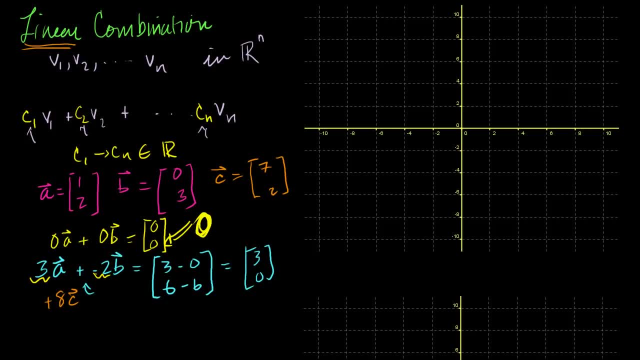 that confounds. I think it's just the very nature that it's taught Over here. I just kept putting different numbers for the weights. I guess we could call them for c1 and c2 in this combination of a and b. 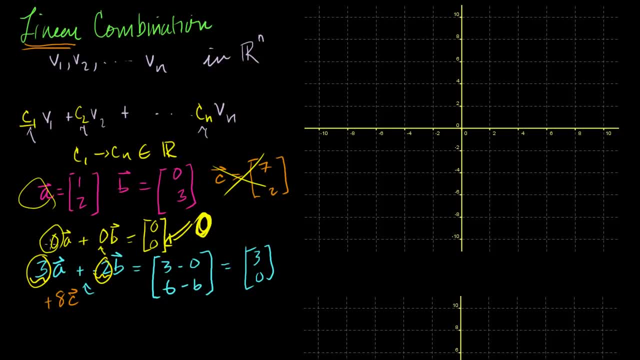 Let's ignore c for a little bit. I just put in a bunch of different numbers there. But it begs the question: what is the set of all of the vectors I could have created? And this is just one member of that set. But what is the set of all of the vectors I could have? 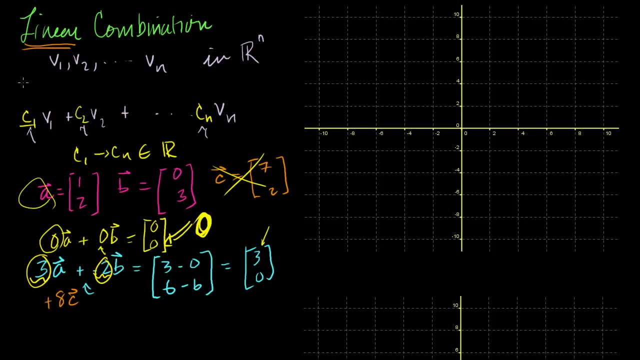 created by taking linear combinations of a and b. So let me draw a and b here. Maybe we could think about it visually and then maybe we could think about it mathematically. So let's say a and b, So a is 1, 2.. 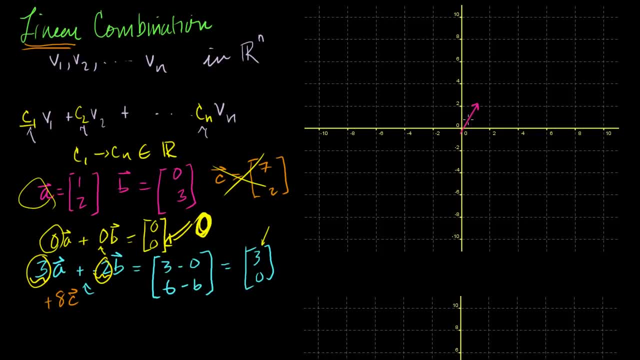 So 1, 2 looks like that. That's vector a. Let me do vector b in a different color. Let me do it in yellow. Vector b is 0, 3.. So vector b looks like that: 0, 3.. 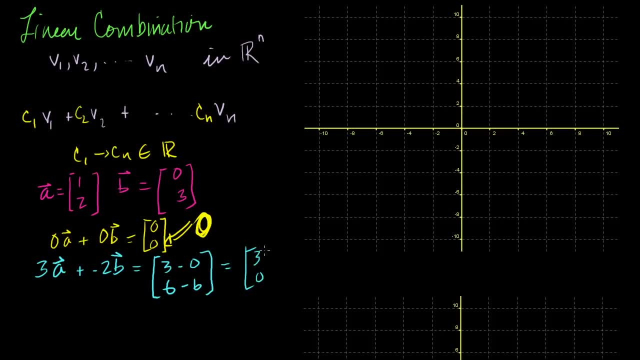 So it's the vector 3,, 0.. This is a linear combination of a and b. I could keep putting in a bunch of random real numbers here and here and I'll just get a bunch of different linear combinations of my vectors a and b. 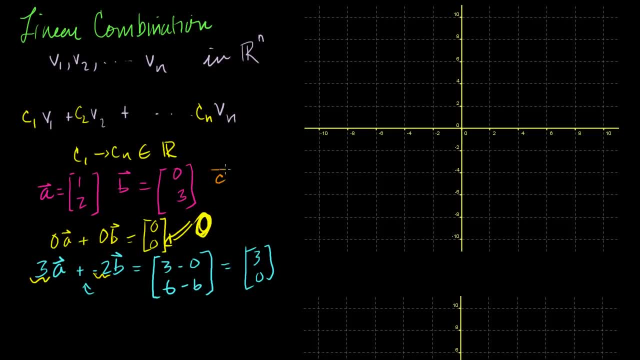 If I had a third vector here, if I had vector c- and maybe that was just 7, 2, then I could add that to the mix and I could throw in plus 8 times vector c. These are all just linear combinations. 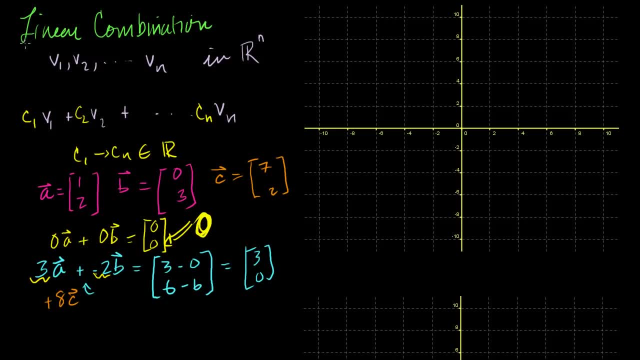 Now why do we just call them combinations? Why do we have to add that little linear prefix there? Because we're just scaling them up. We're not multiplying the vectors times each other. We haven't even defined what it means. It means to multiply a vector and there's actually several. 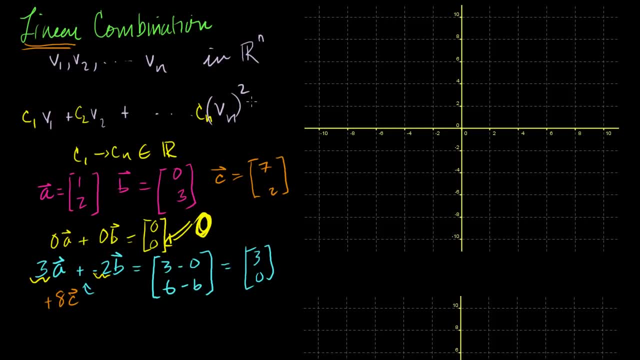 ways to do it, But we can't square a vector, and we haven't even defined what this means yet. but this would all of a sudden make it nonlinear in some form. So all we're doing is we're adding the vectors and we're 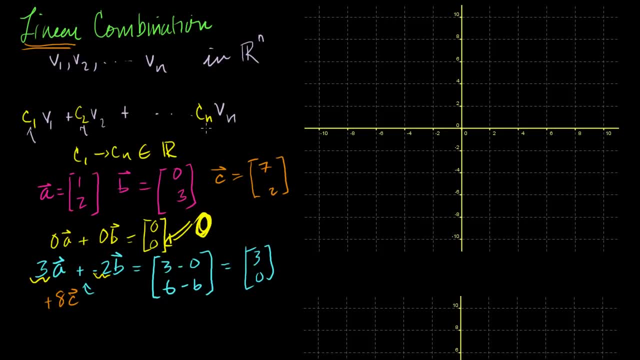 just scaling them up by some scaling factor. So that's why it's called a linear combination. Now you might say: hey Sal, why are you even introducing this idea of a linear combination? Because I want to introduce the idea and this is an idea. 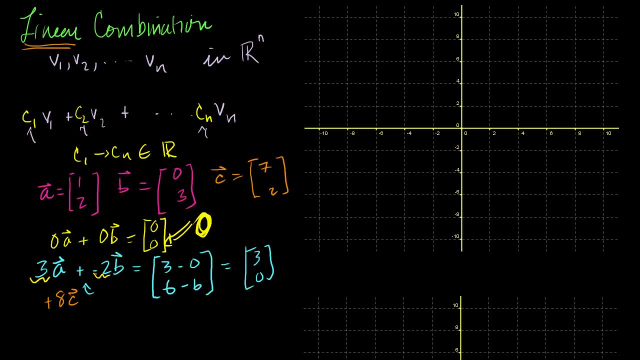 that confounds. I think it's just the very nature that it's taught Over here. I just kept putting different numbers for the weights. I guess we could call them for c1 and c2 in this combination of a and b. 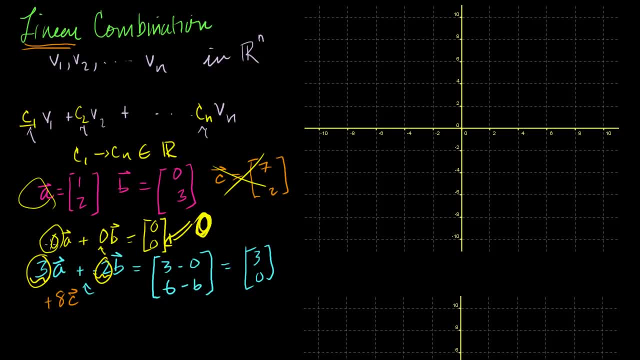 Let's ignore c for a little bit. I just put in a bunch of different numbers there. But it begs the question: what is the set of all of the vectors I could have created? And this is just one member of that set. But what is the set of all of the vectors I could have? 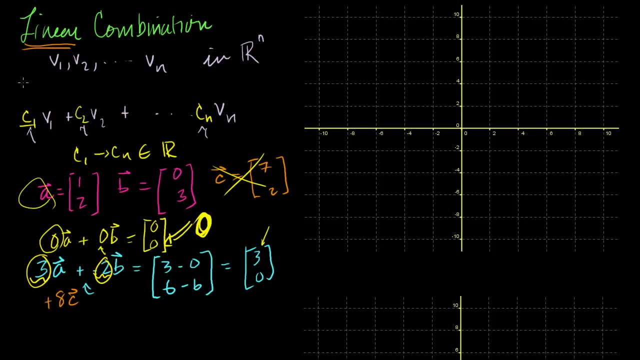 created by taking linear combinations of a and b. So let me draw a and b here. Maybe we could think about it visually and then maybe we could think about it mathematically. So let's say a and b, So a is 1, 2.. 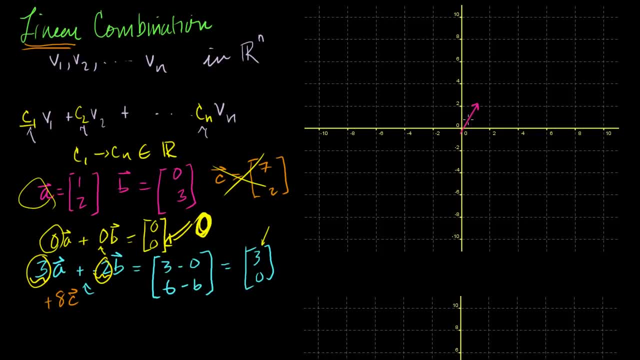 So 1, 2 looks like that. That's vector a. Let me do vector b in a different color. Let me do it in yellow. Vector b is 0, 3.. So vector b looks like that: 0, 3.. 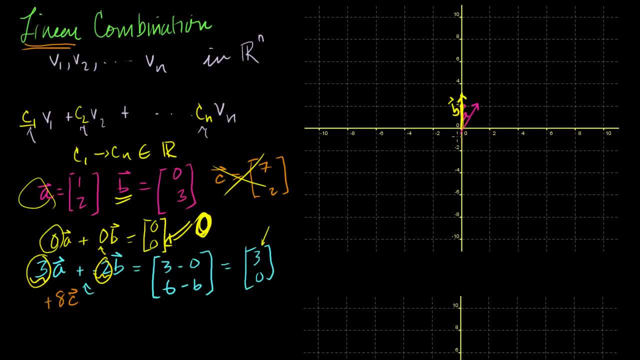 So what's the set of all of the vectors that I can represent? by adding and subtracting these vectors And we saw, if we multiply them both by 0 and add them to each other, we end up there. If we take 3 times a, that's the equivalent of scaling up a. 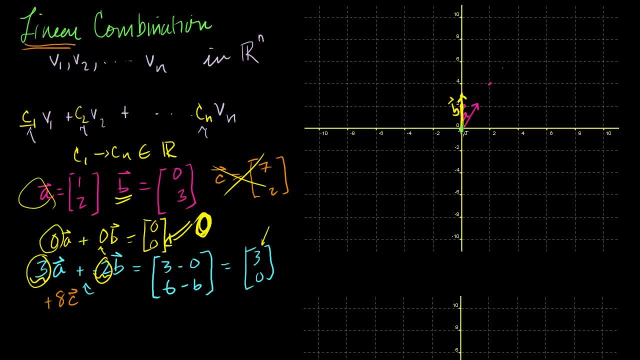 by 3.. So you go 1a, 2a, 3a, So that's 3a 3 times a will look like that. So this vector is 3a, And then we add it to that 2b. 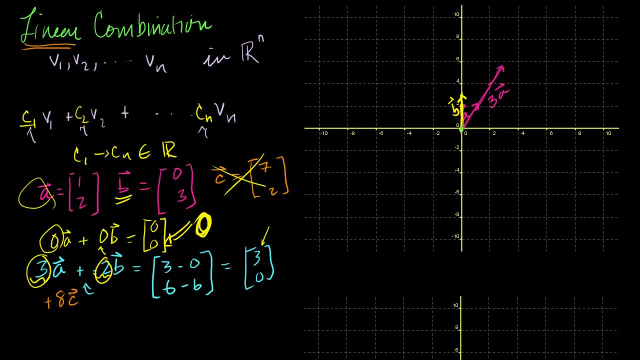 Oh no, We subtracted 2b from that, So minus b looks like this. Minus 2b looks like this. This is minus 2b All the way. in standard form. standard position: Minus 2b. 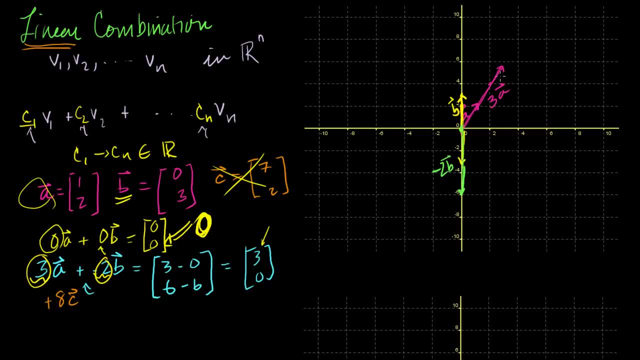 So if you add 3a to minus 2b, we get to this vector: 3a to minus 2b, You get this vector right here, And that's exactly what we did when we solved it mathematically: You get the vector 3, 0.. 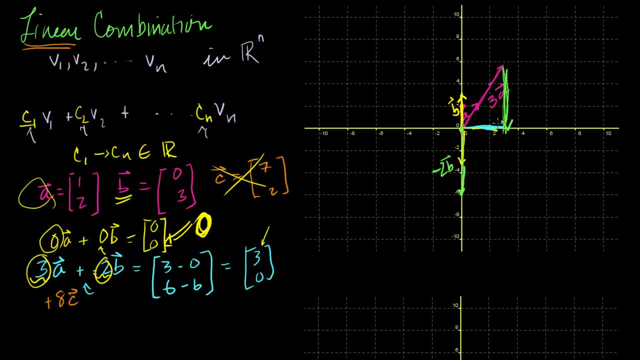 You get this vector right here: 3,, 3,, 0. But this was just one combination, one linear combination of a and b. I could have, instead of multiplying a times 3, I could have multiplied a times 1 and 1 half and just gotten right. 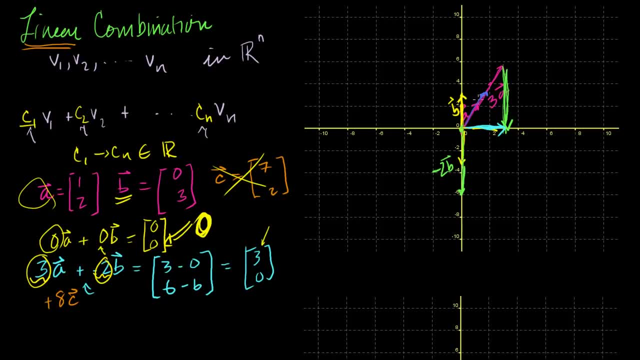 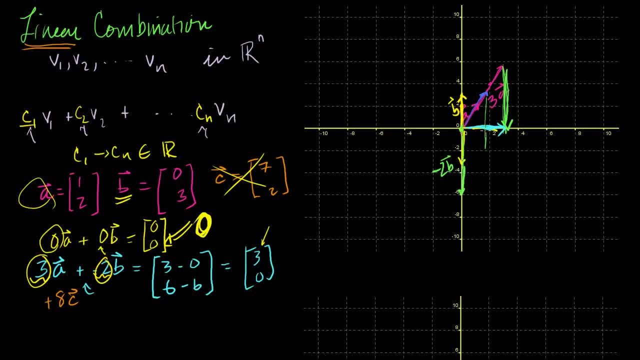 Minus 2b would still look the same. It would look like something like this. It would look something like this, And so our new vector that we would find would be something like this. So I just showed you I could find this vector with a linear combination. 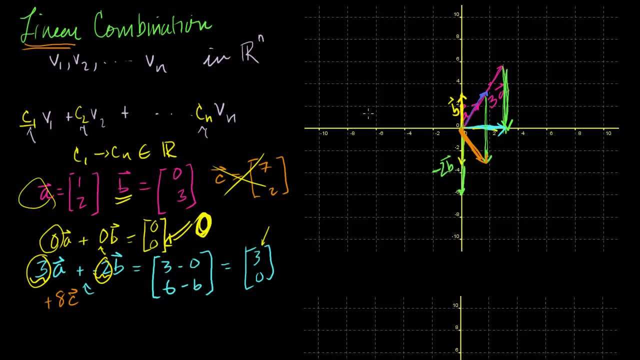 I could find this vector with a linear combination And it actually turns out that you can represent any vector in R2 with some linear combination of these vectors right here, a and b, And let's just think of an example, or maybe just try a. 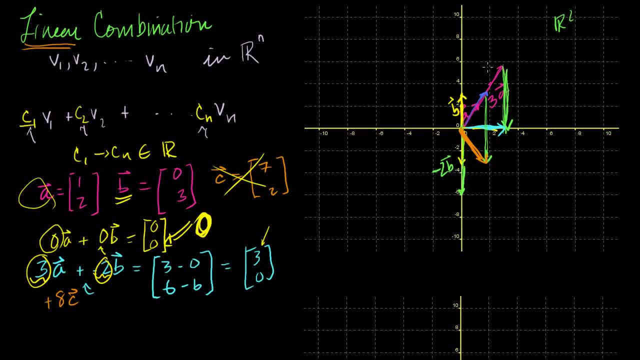 mental visual example: Wherever we want to go, we could go arbitrarily. We could scale a up by some arbitrary value. So this is some scaled up, So this is some weight on a, And then we can add up arbitrary multiples of b. 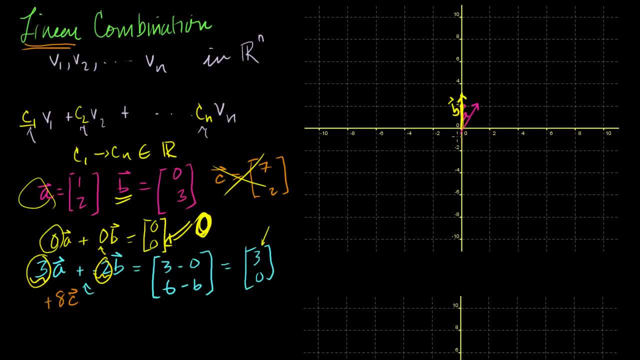 So what's the set of all of the vectors that I can represent? by adding and subtracting these vectors And we saw, if we multiply them both by 0 and add them to each other, we end up there. If we take 3 times a, that's the equivalent of scaling up a. 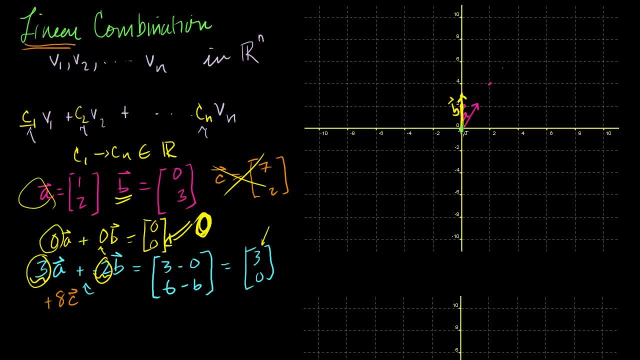 by 3.. So you go 1a, 2a, 3a, So that's 3a 3 times a will look like that. So this vector is 3a, And then we add it to that 2b. 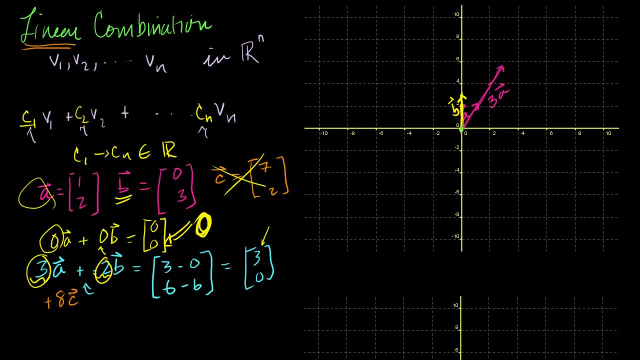 Oh no, We subtracted 2b from that, So minus b looks like this. Minus 2b looks like this. This is minus 2b All the way. in standard form. standard position: Minus 2b. 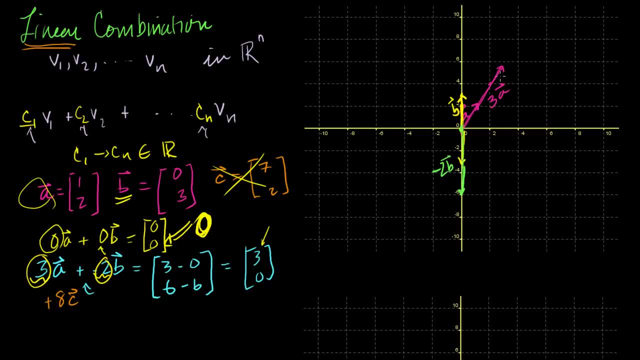 So if you add 3a to minus 2b, we get to this vector: 3a to minus 2b, You get this vector right here, And that's exactly what we did when we solved it mathematically: You get the vector 3, 0.. 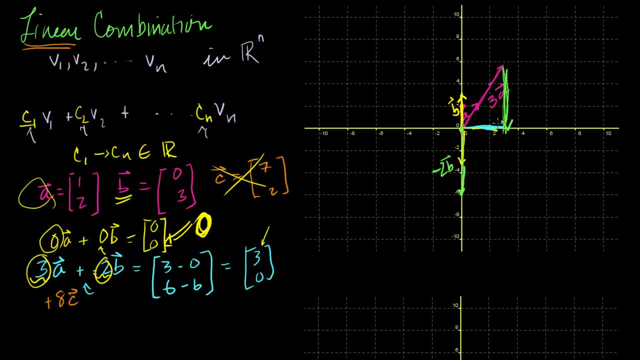 You get this vector right here: 3,, 3,, 0. But this was just one combination, one linear combination of a and b. I could have, instead of multiplying a times 3, I could have multiplied a times 1 and 1 half and just gotten right. 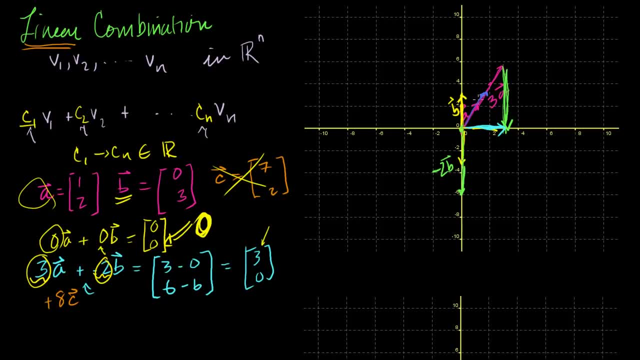 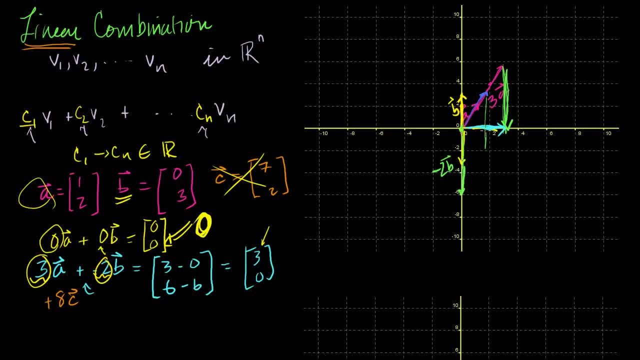 Minus 2b would still look the same. It would look like something like this. It would look something like this, And so our new vector that we would find would be something like this. So I just showed you I could find this vector with a linear combination. 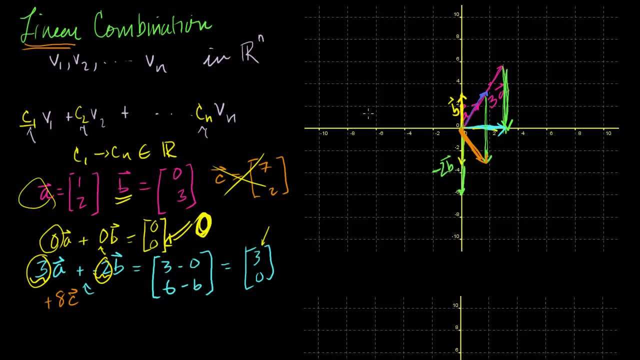 I could find this vector with a linear combination And it actually turns out that you can represent any vector in R2 with some linear combination of these vectors right here, a and b, And let's just think of an example, or maybe just try a. 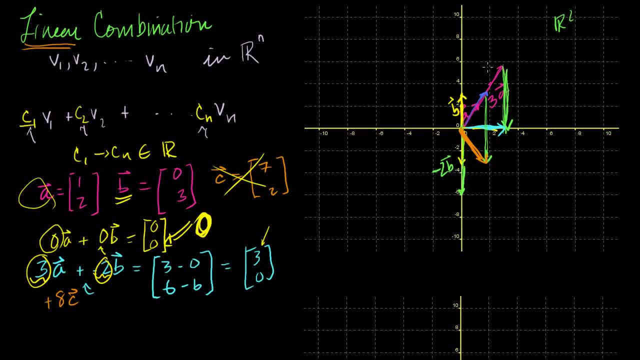 mental visual example: Wherever we want to go, we could go arbitrarily. We could scale a up by some arbitrary value. So this is some scaled up, So this is some weight on a, And then we can add up arbitrary multiples of b. 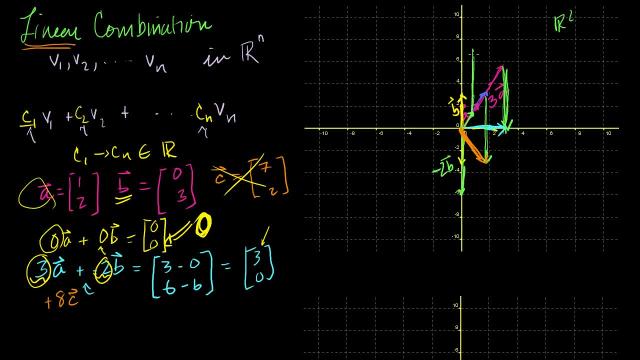 b goes straight up and down. So we could add up arbitrary multiples of b to that. So we could get any point on this vector, on this line, right there. Now, if we scaled a up a little bit more and then added any multiple b, we'd get anything on that line. 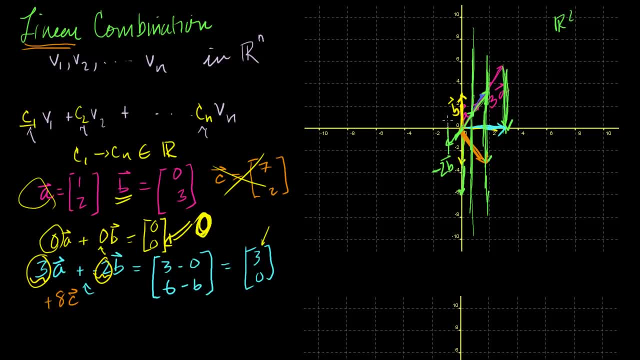 If we multiplied a times a negative number and then added a- b in either direction, we'd get anything on that line. We can keep doing that And there's no reason why we can't pick an arbitrary a that can fill in any of these gaps. 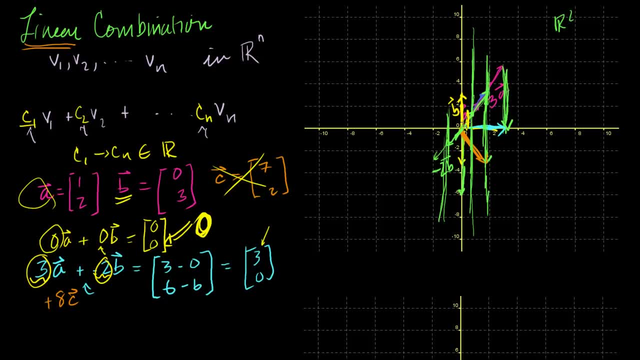 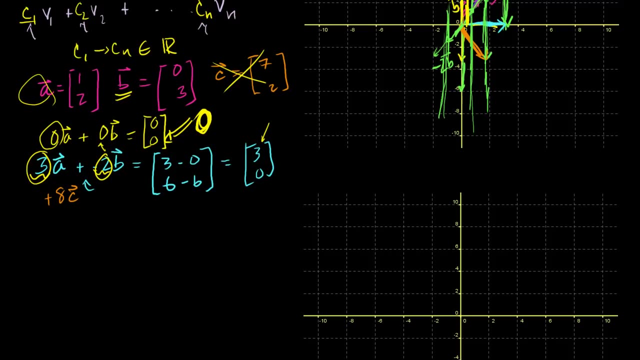 If we want a point here, we just take a little smaller a and then we can add all the b's that fill up all of that line. So we could fill up any point in R2 with the combinations of a and b. So what we can write here is that the span of the vectors a 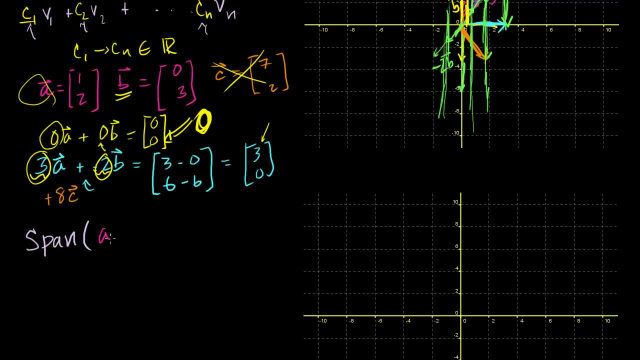 and b, it equals R2, or it equals all the vectors in R2, which is all the tuples. R2 is all the tuples Made of two ordered tuples of two real numbers, So it equals all of R2.. This just means that I can represent any vector in R2. 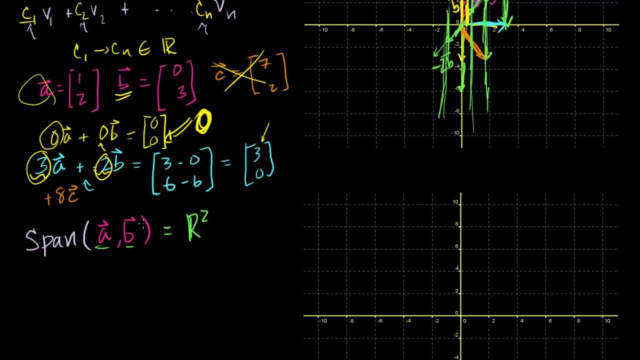 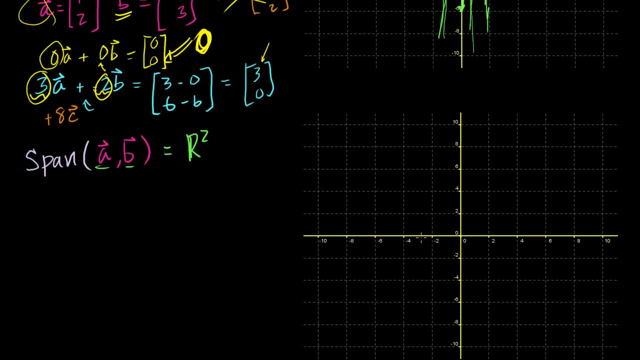 with some linear combination of a and b And you're like, hey, can't I do that with any two vectors. Well, what if a and b were the vector? Let's say the vector 2, 2 was a, So a is equal to 2, 2.. 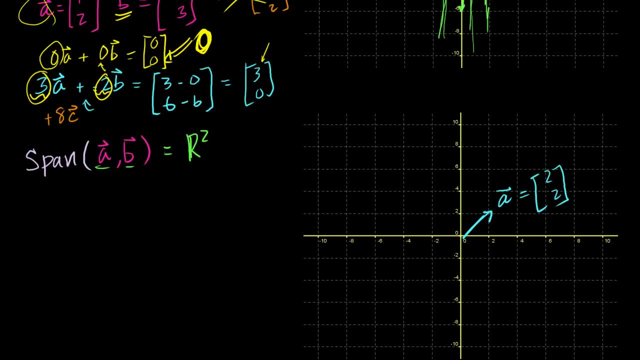 And let's say that b is the vector minus 2.. So b is that vector. So b is the vector minus 2, minus 2.. Now can I represent any vector with these? Well, I can scale a up and down. 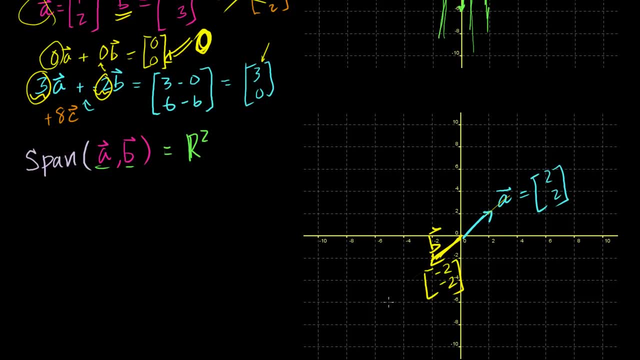 So I can scale a up and down to get anywhere on this line And then I can add b or anywhere to it And b is essentially going in the same direction. It's just in the opposite direction. But I can multiply it by negative. 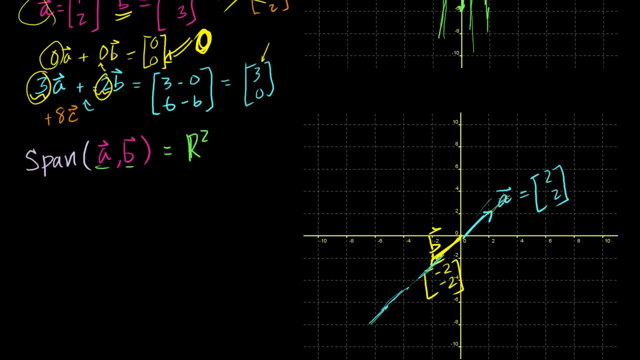 and go anywhere in the line. So any combination of a and b will just end up on this line right here. if I draw it in standard form, It'll be in. It'll be a vector with the same slope as either a or b. 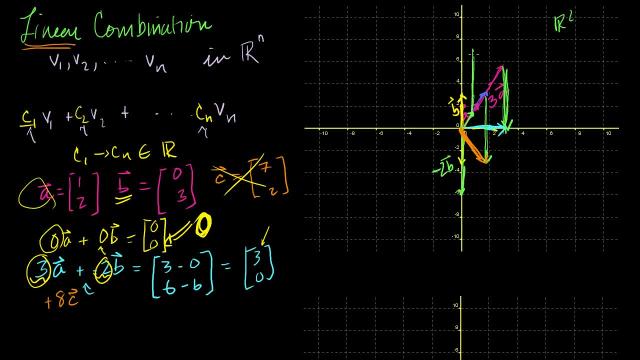 b goes straight up and down. So we could add up arbitrary multiples of b to that. So we could get any point on this vector, on this line, right there. Now, if we scaled a up a little bit more and then added any multiple b, we'd get anything on that line. 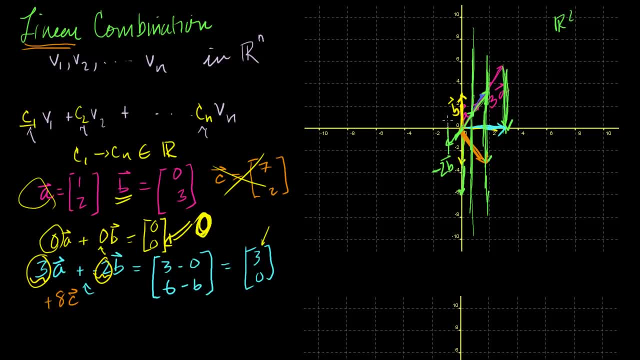 If we multiplied a times a negative number and then added a- b in either direction, we'd get anything on that line. We can keep doing that And there's no reason why we can't pick an arbitrary a that can fill in any of these gaps. 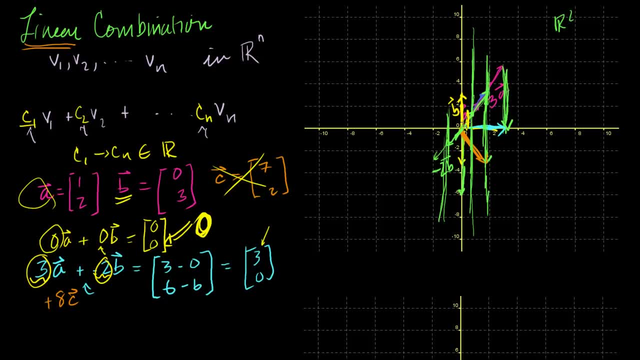 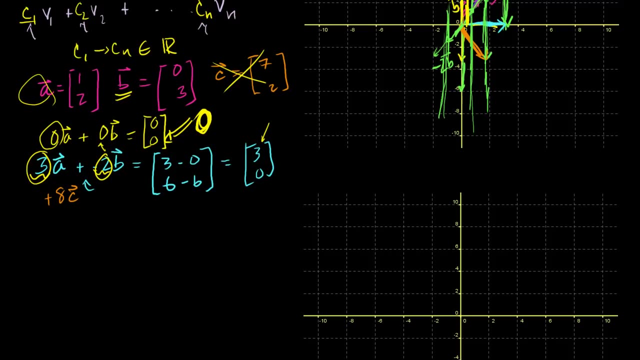 If we want a point here, we just take a little smaller a and then we can add all the b's that fill up all of that line. So we could fill up any point in r2 with the combinations of a and b. So what we can write here is that the span of the vectors a 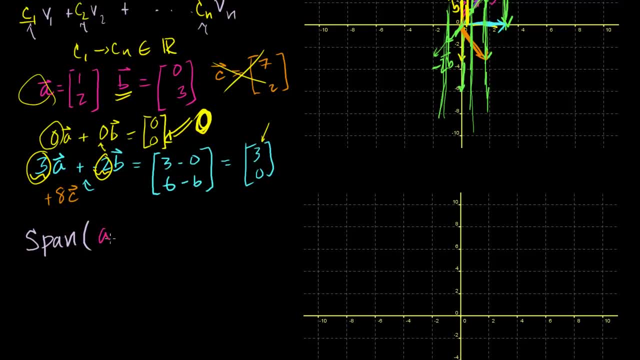 and b, it equals r2.. Or it equals all the vectors in r2, which is all the tuples. r2 is all the tuples Made of two ordered tuples of two real numbers, So it equals all of r2.. This just means that I can represent any vector in r2. 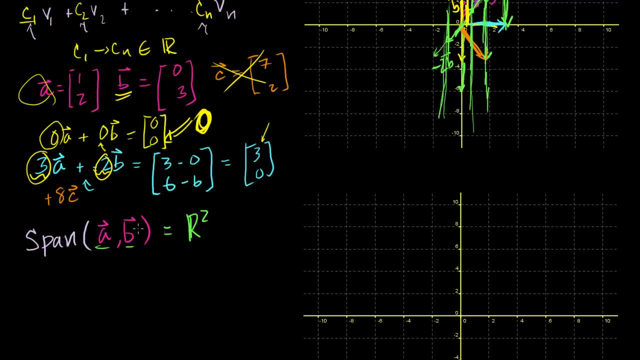 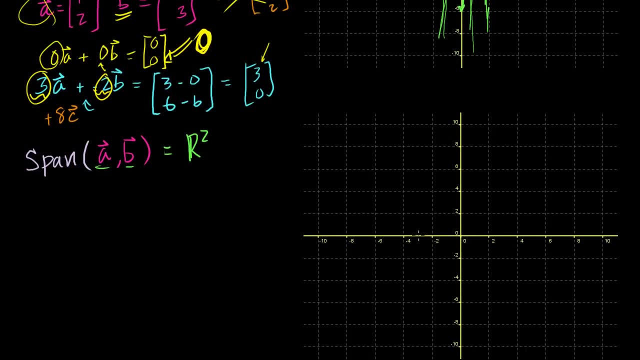 with some linear combination of a and b And you're like, hey, can't I do that with any two vectors. Well, what if a and b were the vector? Let's say the vector 2, 2 was a, So a is equal to 2, 2.. 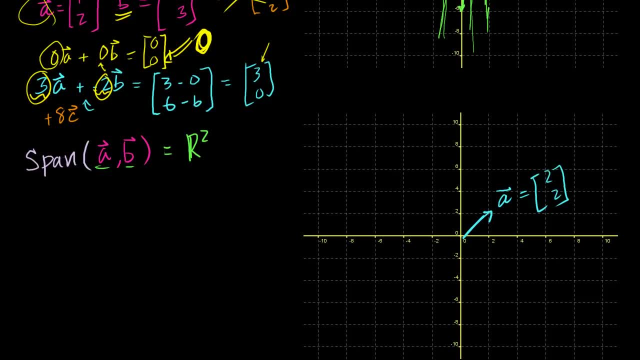 And let's say that b is the vector minus 2.. Minus 2, minus 2.. So b is that vector. So b is the vector minus 2, minus 2.. Now can I represent any vector with these? 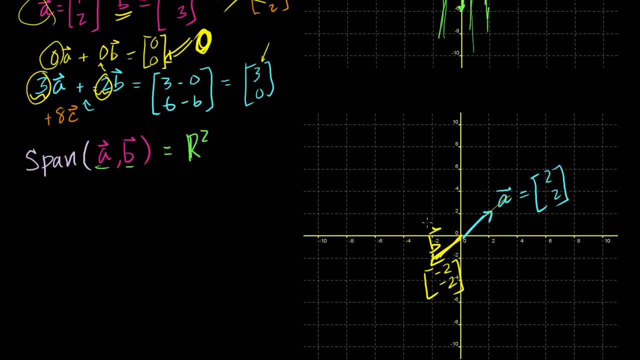 Well, I can scale a up and down. So I can scale a up and down to get anywhere on this line, And then I can add b or anywhere to it, And b is essentially going in the same direction. It's just in the opposite direction. 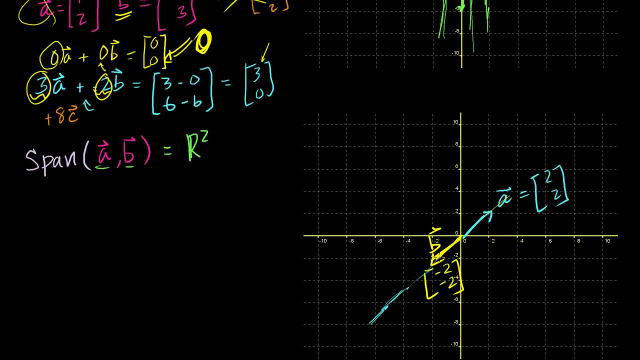 But I can multiply it by negative and go anywhere in the line. So any combination of a and b will just end up on this line right here. if I draw it in standard form, It'll be a vector with the same slope as either a or b. 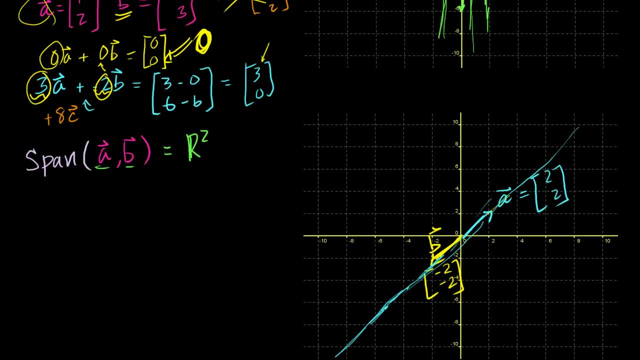 or same inclination, whatever you want to call it. There's no combination of a and b that I could represent this vector. I could represent vector c, I just can't do it. I can add in standard form, I could just keep adding: scale up a, scale up b, put them. 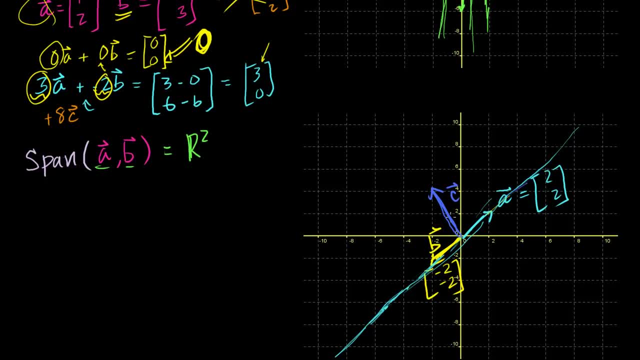 heads to tails. I'll just get to stuff on this line. I'll never get to this. So in this case, the span- and I want to be clear- this is for this particular a and b, not for the a and b. 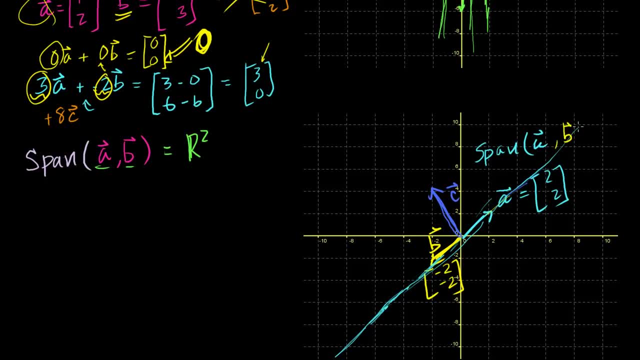 For this blue a and this yellow b. the span here is just this line. It's just this line. It's not all of R2.. So this isn't just some kind of statement You might have. when I first did it with that example, I 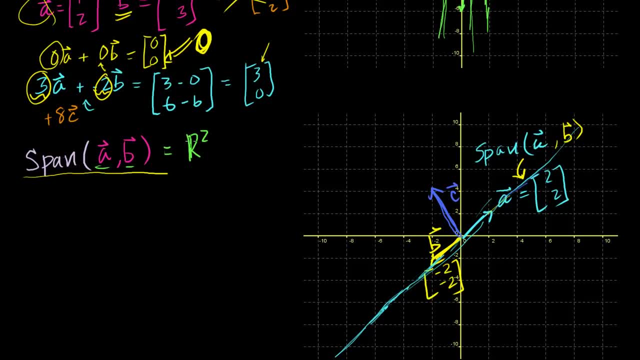 was like: oh, any two vectors can I represent? Can any two vectors represent anything in R2?? Well no, I just showed you two vectors. It can't represent that. And what, if? I mean, you know what is the span of what is? 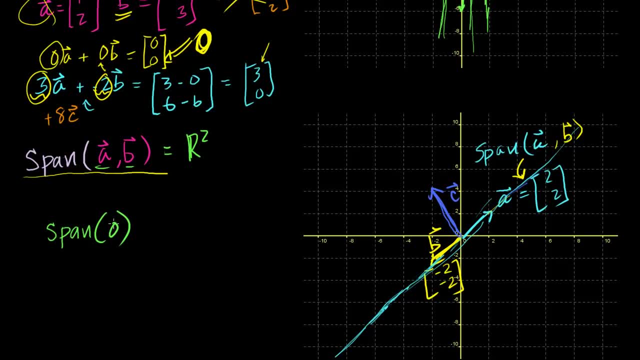 the span, The span of the 0 vector. I'll put even a cap over it- The 0 vector. I make it really bold. Well, the 0 vector is just 0, 0. So I don't care what multiple I put on it. 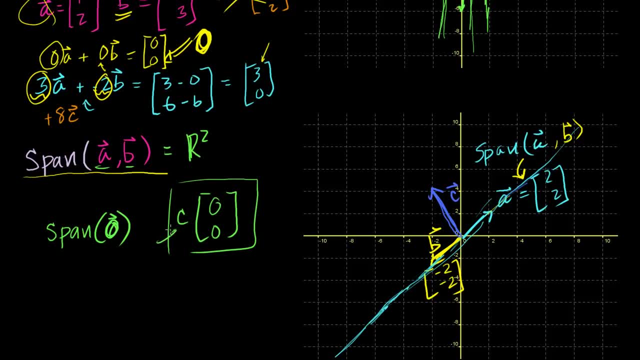 The span of it is all of the linear combinations of this. So essentially I could put arbitrary real numbers here, but I'm just going to end up with the 0, 0 vector. So the span of the 0 vector is just the 0 vector. 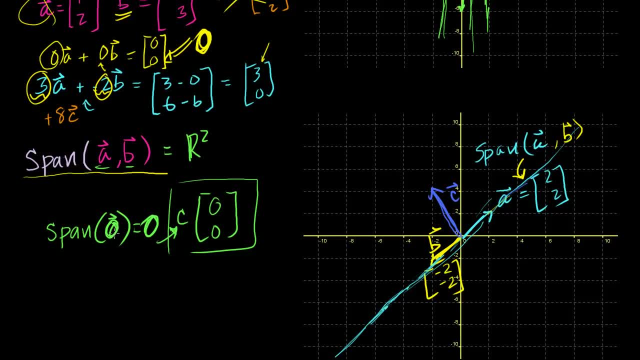 The only vector I can get with a linear combination of this, the 0 vector by itself is just the 0 vector itself. Likewise, if I take the span of just, you know, let's say I go to this, let's say I go back to this example right here. 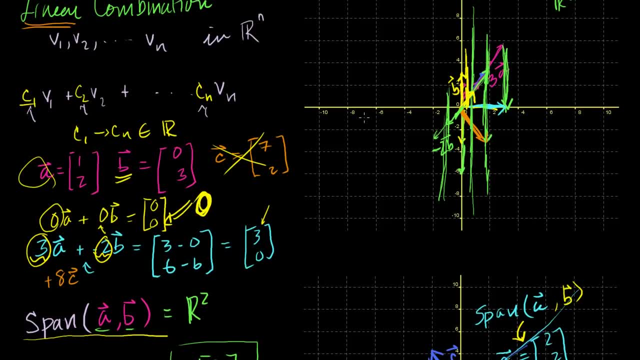 My a vector was right like that. Let me draw it in a better color. My a vector looked like that If I were to ask just what the span of a is. it's all the vectors you can get by creating a linear combination of just a. 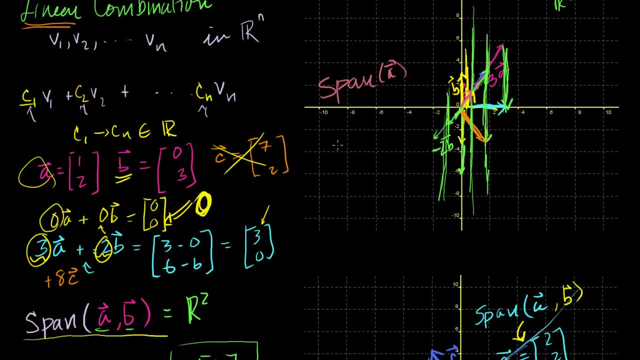 So it's really just scaling. You can't even talk about combinations really, So it's just c times a, all of those vectors. And we saw in the video where I parametricized or showed a parametric representation of a line, that this the span of. 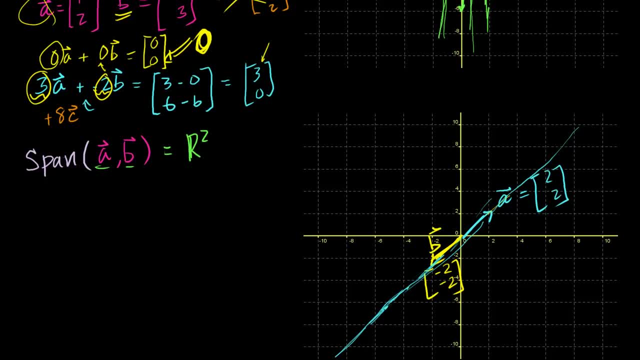 or same inclination, whatever you want to call it. There's no combination of a and b that I could represent this vector. I could represent vector c, I just can't do it. I can add in standard form, I could just keep adding: scale up a, scale up b, put them. 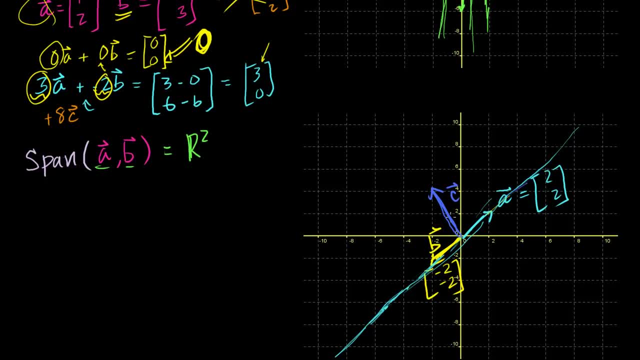 heads to tails. I'll just get to stuff on this line. I'll never get to this. So in this case, the span- and I want to be clear- this is for this particular a and b, not for the a and b. 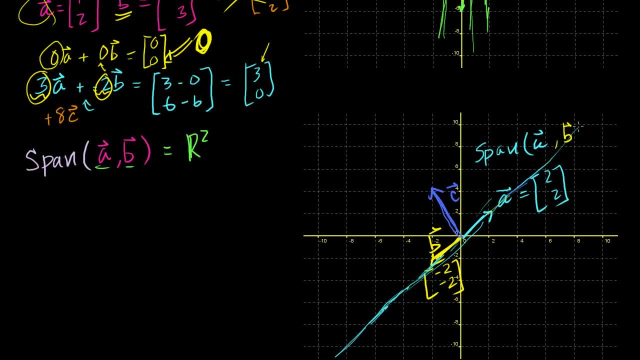 For this blue a and this yellow b. the span here is just this line. It's just this line. It's not all of R2.. So this isn't just some kind of statement You might have. when I first did it with that example, I 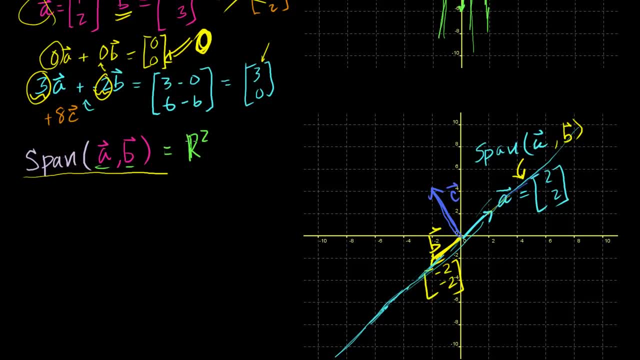 was like: oh, any two vectors can I represent? Can any two vectors represent anything in R2?? Well no, I just showed you two vectors. It can't represent that. And what, if? I mean, what is the span of? 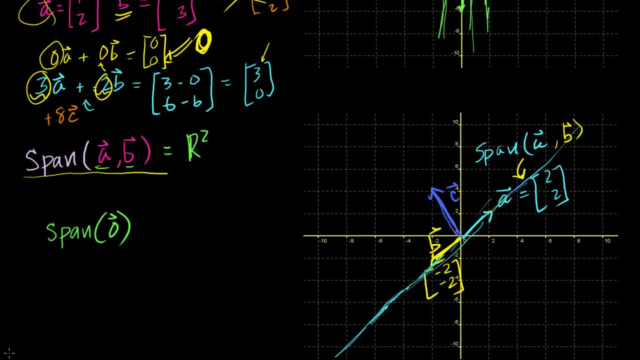 The span of the 0 vector. I'll put even a cap over it. The 0 vector. I make it really bold. Well, the 0 vector is just 0, 0. So I don't care what multiple I put on it. 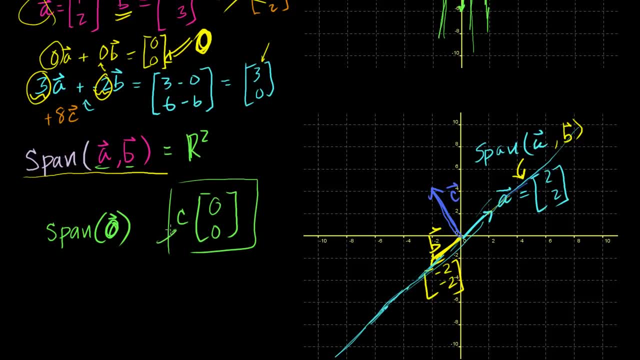 The span of it is all of the linear combinations of this. So essentially I could put arbitrary real numbers here, but I'm just going to end up with the 0, 0 vector. So the span of the 0 vector is just the 0 vector. 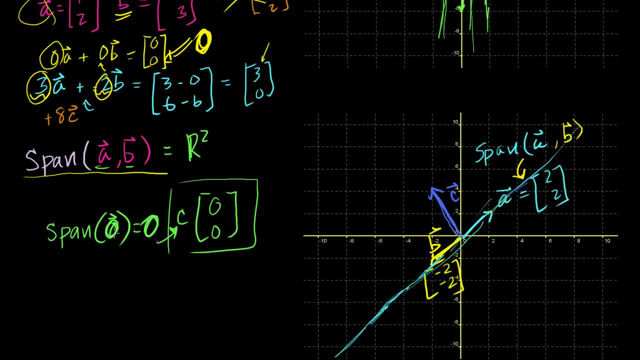 The only vector I can get with a linear combination of this: the 0 vector by 1.. The vector by itself is just the 0 vector itself. Likewise, if I take the span of just, let's say, I go back to this example right here- 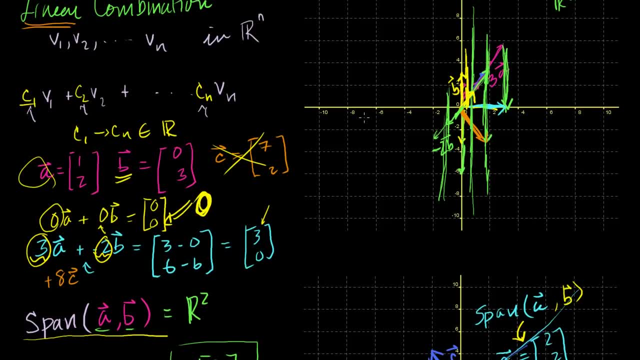 My a vector was right like that. Let me draw it in a better color. My a vector looked like that If I were to ask just what the span of a is. it's all the vectors you can get by creating a linear combination of just a. 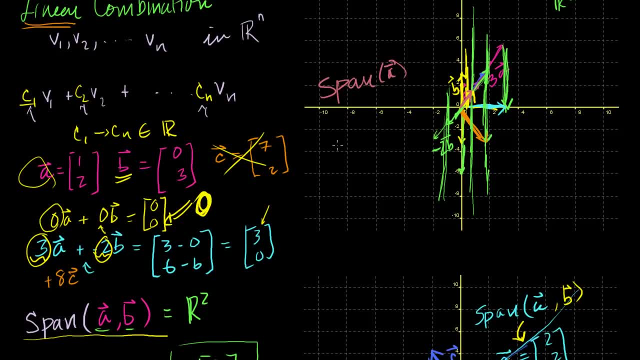 So it's really just scaling. You can't even talk about combinations really, So it's just c times a, all of those vectors. And we saw in the video where I parametricized or showed a parametric representation of a line, that this the span of. 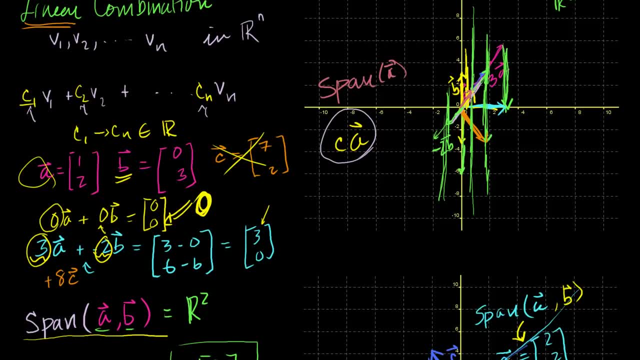 just this vector. a is the line that's formed when you just scale a up and down. So the span of a is just a line. You have to have two vectors, and they can't be collinear, in order to span all of R2.. 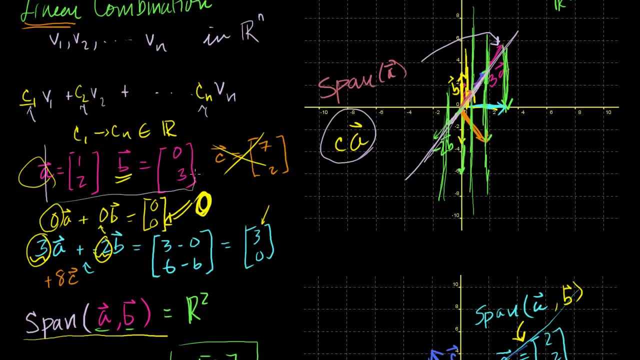 And I haven't proven that to you yet, but we saw with this example, if you pick this a and this b, you can represent all of R2 with just these two vectors, Now, the two vectors that you're most familiar with. that. 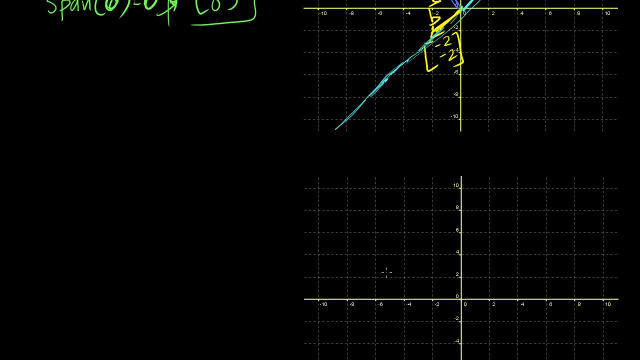 span R2 are: if you take a little physics class, you have your i and j unit vectors And in R notation i, the unit vector i that you learned in physics class would be the vector 1, 0.. So this is i. 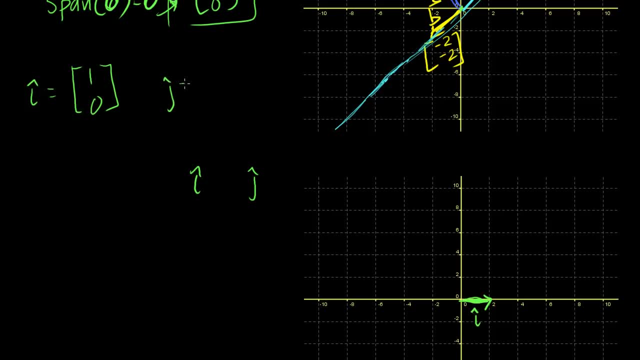 That's the vector i, And then the vector j is the unit vector 0, 1.. This is what you learned in physics class. Let me do it in a different color. This is j. j is that. And you learned that they're orthogonal. 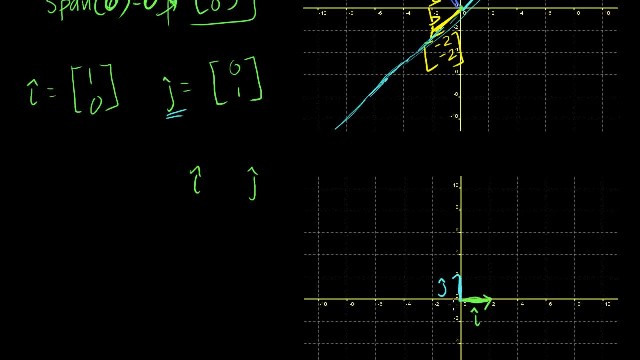 And we're going to talk a lot more about what orthogonality means, But in our traditional sense that we learned in high school, it means that they're 90 degrees. But you can clearly represent any vector in R2 by these two vectors. 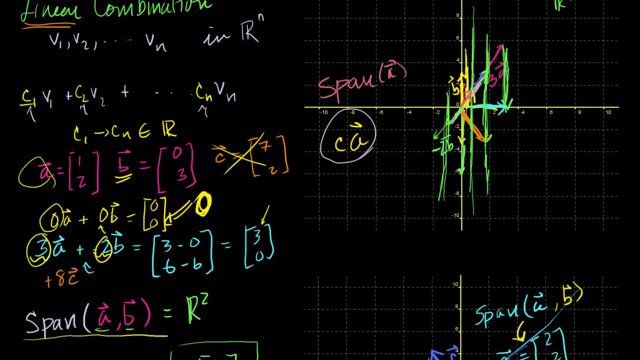 just this vector. a is the line that's formed when you just scale a up and down. So the span of a is just a line. You have to have two vectors, and they can't be collinear, in order to span all of R2.. 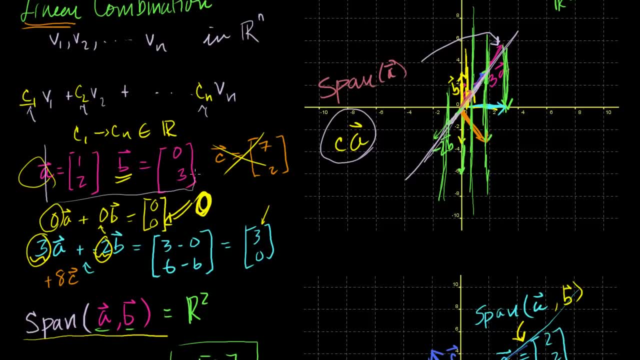 And I haven't proven that to you yet, but we saw with this example, If you pick this a and this b, you can represent all of R2 with just these two vectors, Now, the two vectors that you're most familiar with. that. 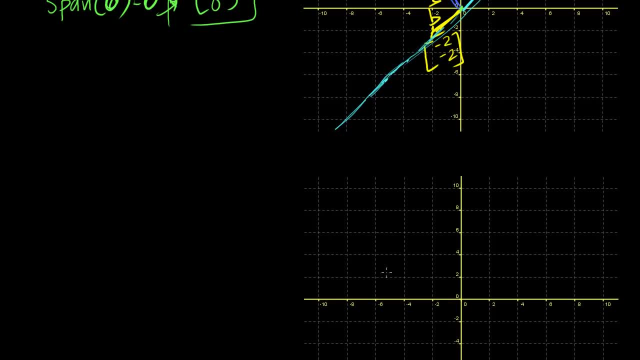 span R2 are: if you take a little physics class, you have your i and j unit vectors And in R, notation i, the unit vector i that you learn in physics class would be the vector 1, 0.. So this is i. 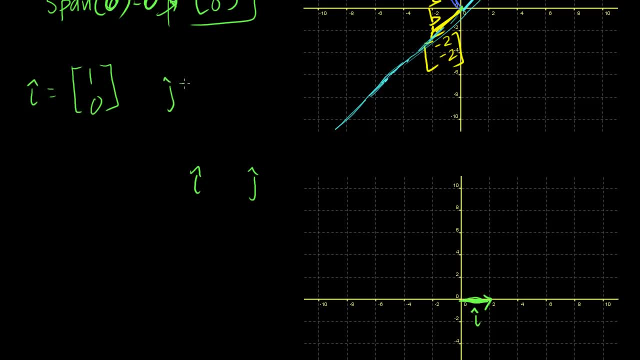 That's the vector i, And then the vector j is the unit vector 0, 1.. This is what you learn in physics class. Let me do it in a different color. This is j. j is that, And you learn that they're orthogonal and we're going to 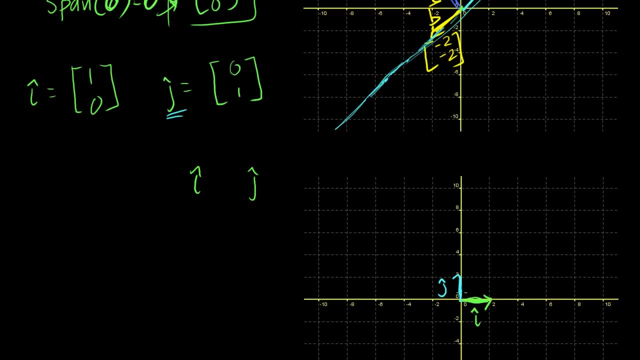 talk a lot more about what orthogonality means, But in our traditional sense that we learned in high school, it means that they're 90 degrees, But you can clearly represent any vector in R2 by these two vectors And the fact that they're orthogonal. 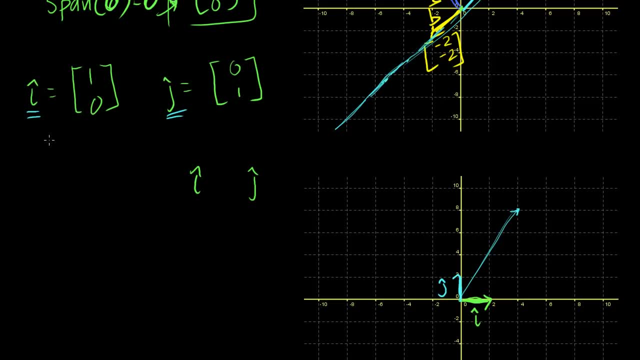 makes them extra nice. And that's why these form- and I'm going to throw out a word here that I haven't defined yet- these form the basis. These form a basis for R2, in that you can represent anything in R2 by these two vectors alone. 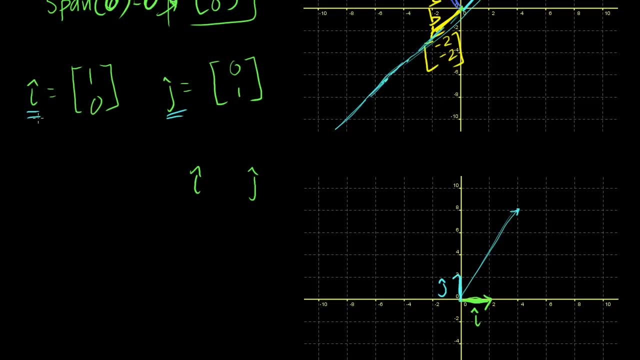 And the fact that they're orthogonal makes them a little bit more obvious, It makes them extra nice, And that's why these form- and I'm going to throw out a word here that I haven't defined yet- these form the basis. These form a basis for R2.. 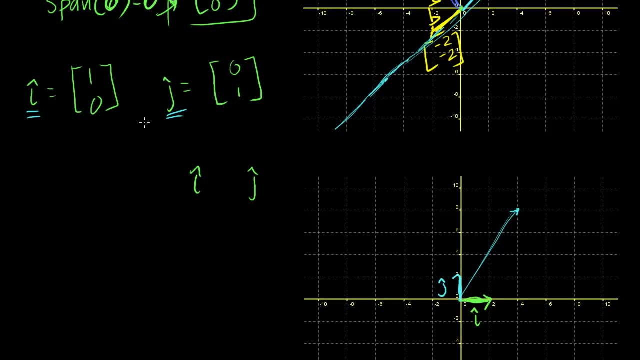 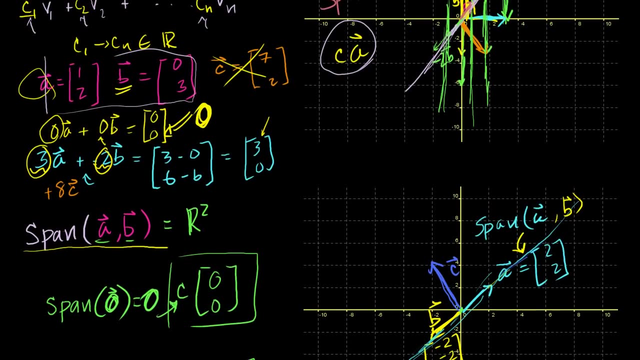 In fact you can represent anything in R2 by these two vectors alone, And I'm not going to even define what basis is. That's going to be a future video, But let me just write the formal mathy definition of span, just so you're satisfied. 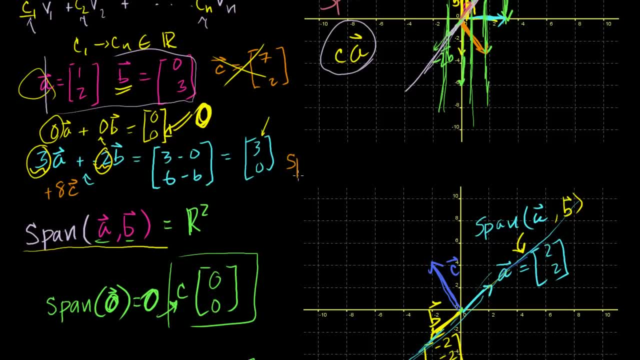 So if I were to write the span of a set of vectors, v1,, v2, all the way to vn, That just means the set of all of the vectors where I have c1 times v1 plus c2 times v2, all the way to cn. let me scroll. 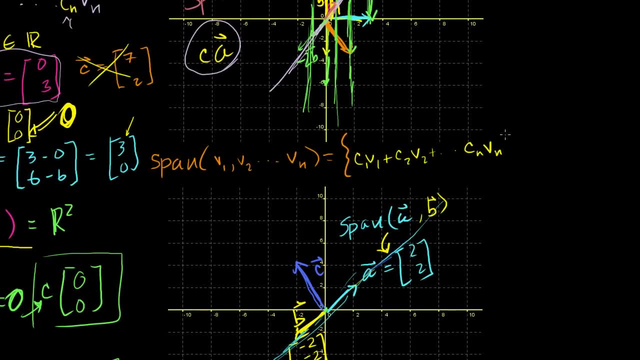 over all the way to cn vn. So this is a set of vectors Because I can pick my ci's to be any member of the real numbers, And that's true for i- Sorry I should write 4i- being anywhere between 1 and n. 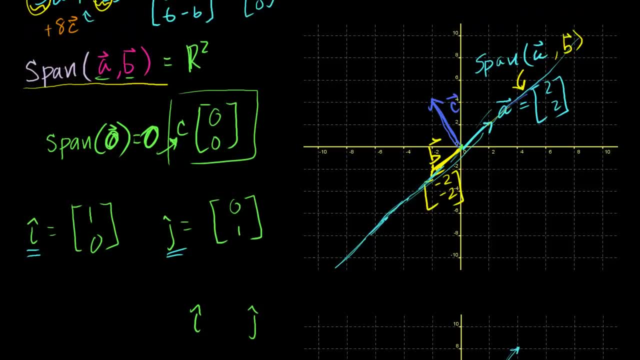 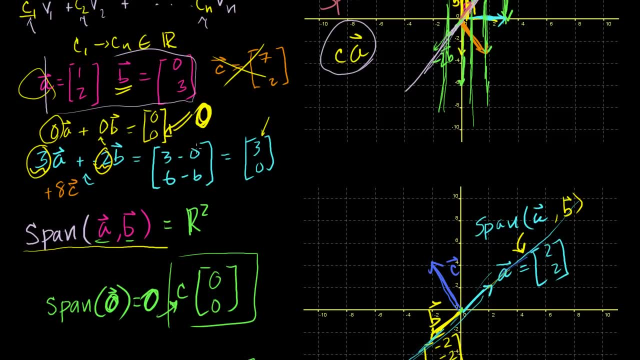 I'm not going to even define what basis is. That's going to be a future video- But let me just write the formal mathy definition of span, just so you're satisfied. So if I were to write the span of a set of vectors- v1,, v2,- 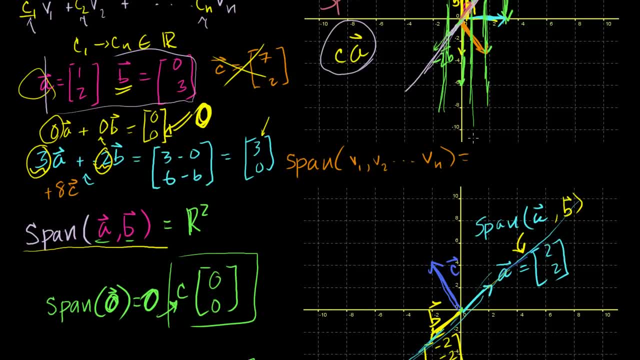 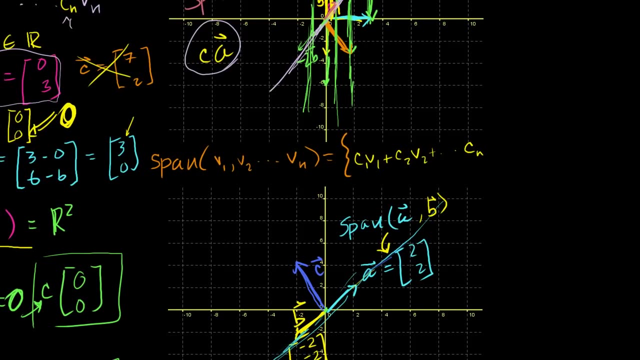 all the way to vn. that just means the set of all of the vectors where I have c1 times v1 plus c2 times v2, all the way to cn. let me scroll over all the way to cn, vn. So this is a set of vectors because I can pick my ci's to. 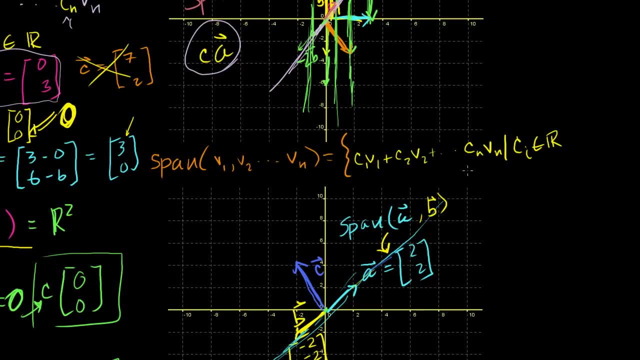 be any member of the real numbers, and that's true for i from, so I should write 4i being anywhere between 1 and n. All I'm saying is is that, look, I can multiply each of these vectors by any value, any arbitrary value, real value. 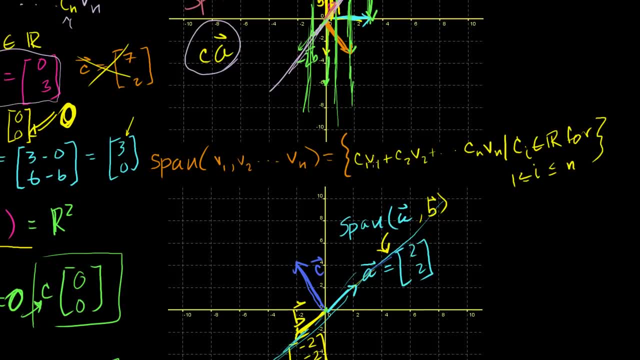 and then I can add them up And now the set of all of the combinations, scaled up combinations I can get. that's the span, That's the span of these vectors. You can kind of view it as the space of all of the vectors. 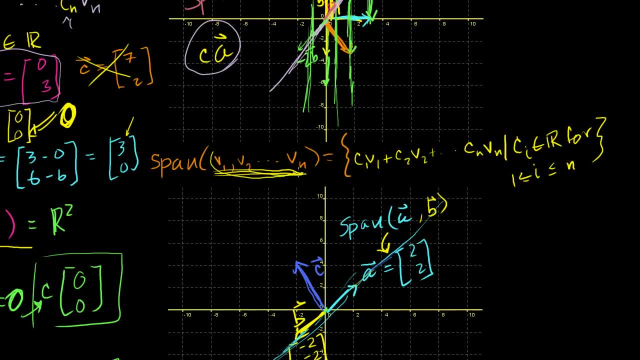 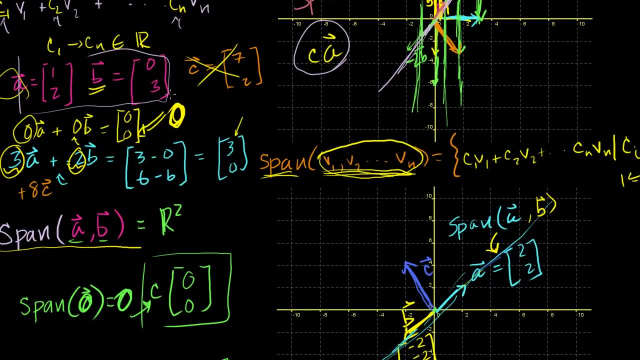 that can be Represented by a combination of these vectors right there. And so the word span. I think it does have an intuitive sense. I mean, if I say that, my first example, I saw that those two vectors span, or a and b, spans r2.. 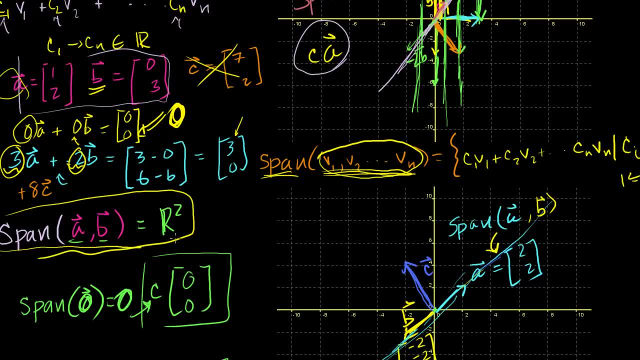 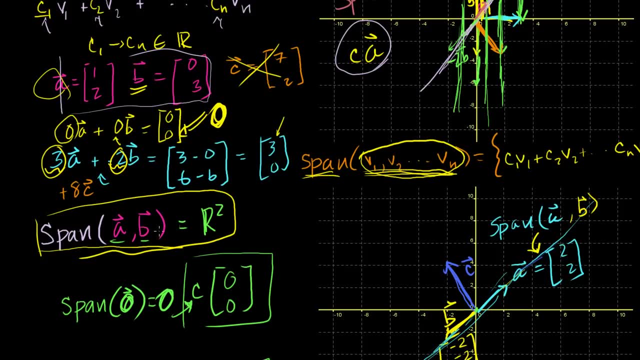 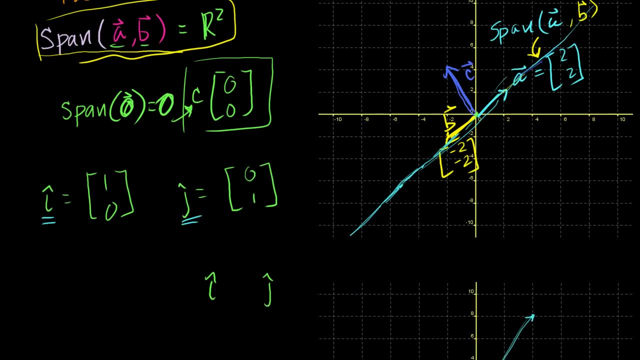 I wrote it right here That tells me that any vector in r2 can be represented by a linear combination of a and b. And actually, just in case That visual Kind of pseudo proof doesn't do you justice, Let me prove it to you algebraically. 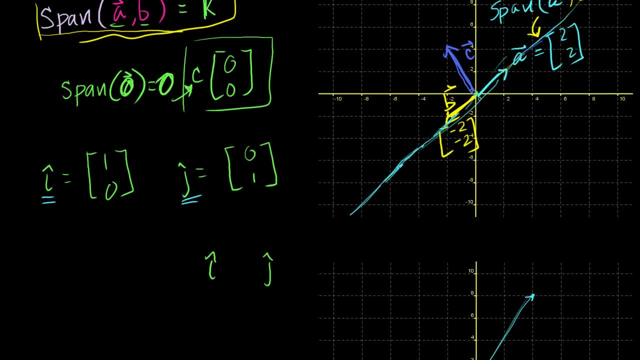 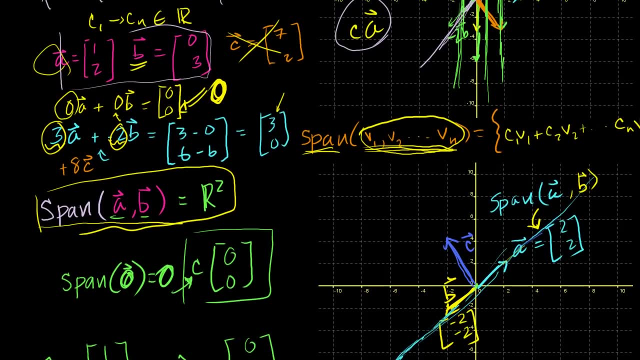 I'm telling you that I can take. Let's say I want to represent. you know I have some. Let me rewrite my a's and b's again. So this was my vector a: It was 1, 2.. And b was 0, 3.. 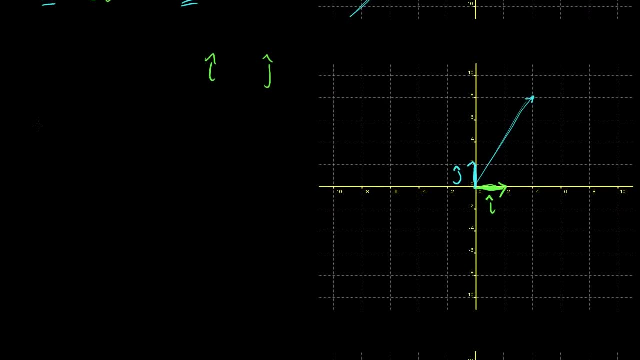 Let me remember that. So my vector a is 1, 2.. And my vector b was 0, 3.. Now my claim was that I can represent any point. Let's say I want to represent some arbitrary point x in r2.. 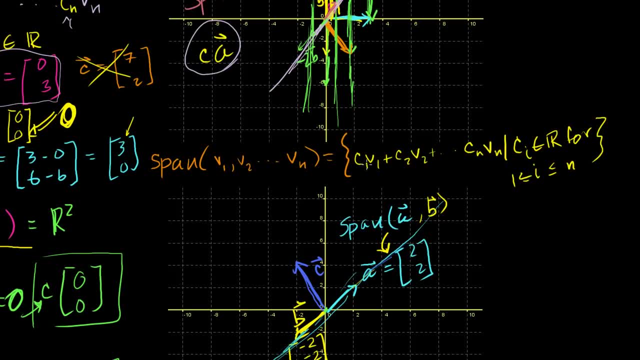 All I'm saying is that, look, I can multiply each of these vectors by any value, any arbitrary value, real value, and then I can add them up. And now the set of all of the combinations scaled up combinations I can get. that's the span of these vectors. 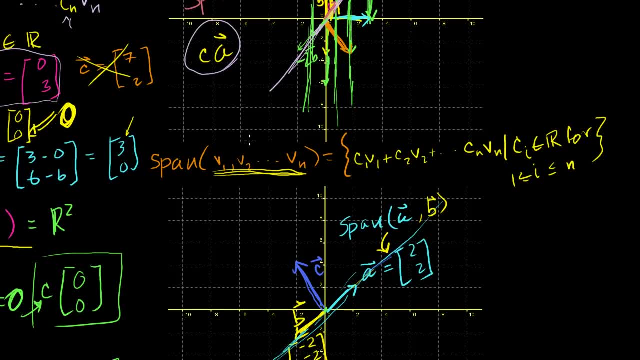 You can kind of view it as the space of all of the vectors that can be represented by a combination. And so the word span. I think it does have an intuitive sense. I mean, if I say that my first example, I saw that those two 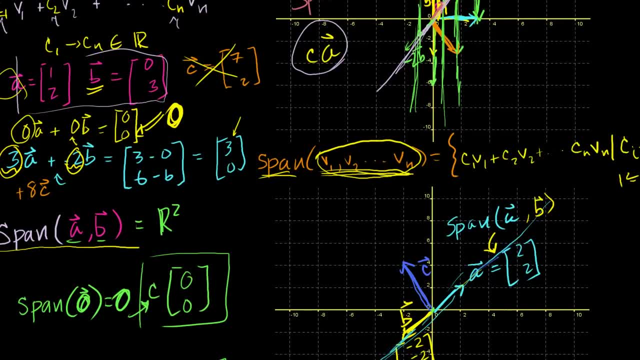 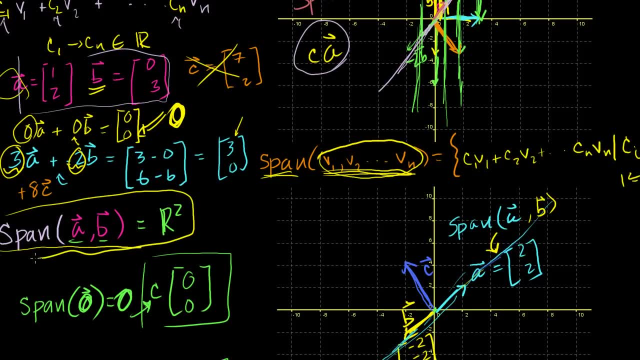 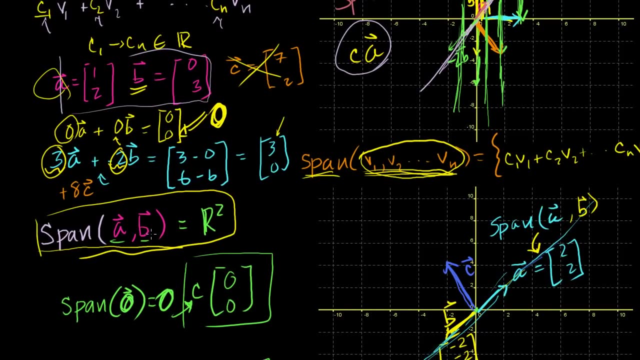 vectors span, or a and b spans, r2.. I wrote it right here. That tells me that any vector in r2 can be represented by a linear combination of a and b. And actually, just in case that visual kind of pseudo proof, I'm going to use a little bit of a little bit of. 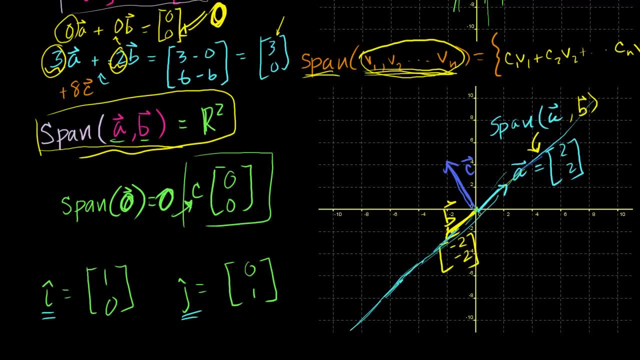 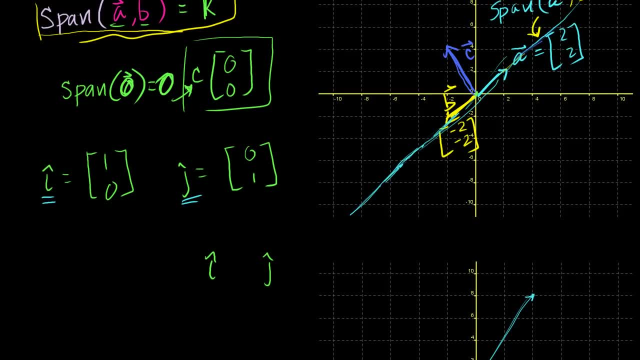 information. If that pseudo proof doesn't do you justice, let me prove it to you algebraically. I'm telling you that I can take. let's say I want to represent you. know I have some. let me rewrite my a's. 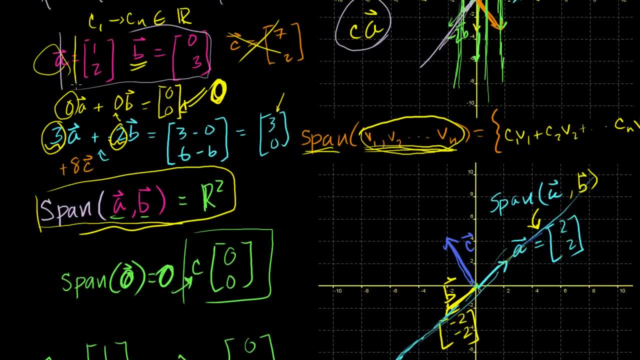 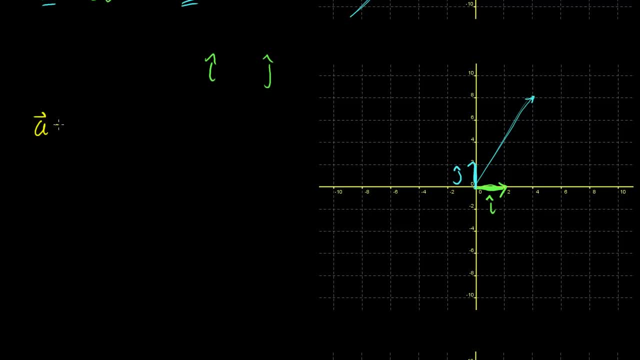 and b's again. So this was my vector a, It was 1,, 2, and b was 0, 3.. Let me remember that. So my vector a is 1, 2, and my vector b was 0, 3.. 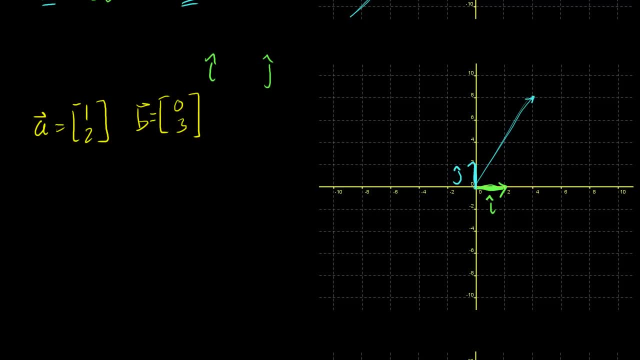 Now My claim was that I could do this. My claim was that I can represent any point. Let's say, I want to represent some arbitrary point x in r2.. So its coordinates are x1 and x2.. I need to be able to prove to you that I can get to any x1. 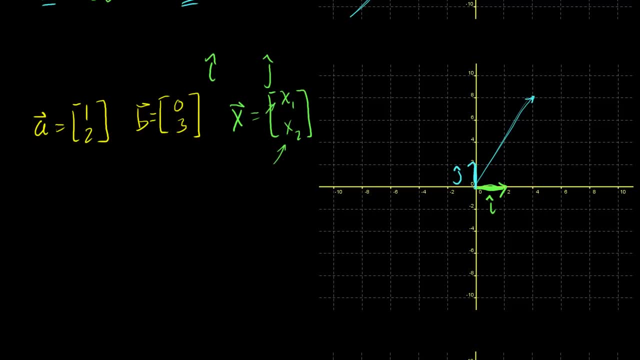 and any x2 with some combination of these guys. So let's say that my combination- I say c1 times a plus c2 times b, has to be equal to my vector x. So let me show you that I can always find a c1 or a c2 given. 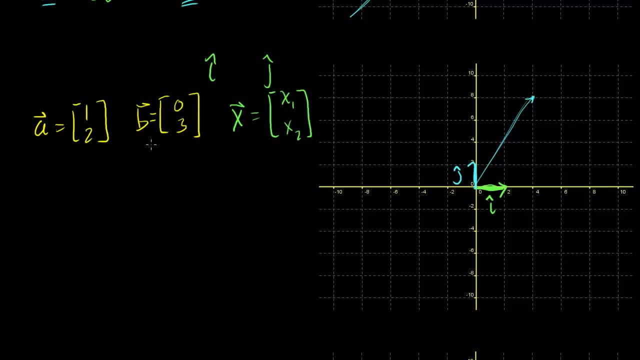 So its coordinates are x1 and x2.. I need to be able to prove to you that I can get to any x1 and any x2 with some combination of these guys. So let's say that my combination. I say c1 times a. 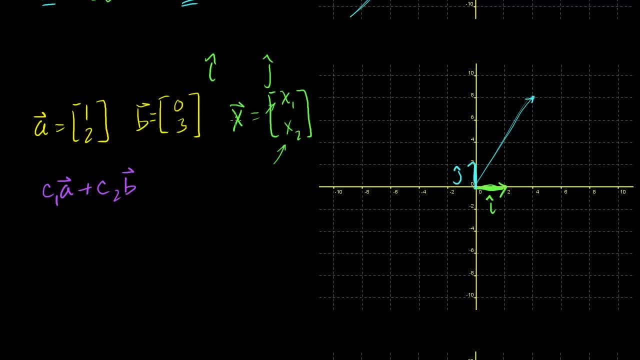 plus c2 times b has to be equal to my vector a. So let me show you that I can always find a c1 or a c2, given that you give me some x's. So let's just write this right here with the actual vectors: 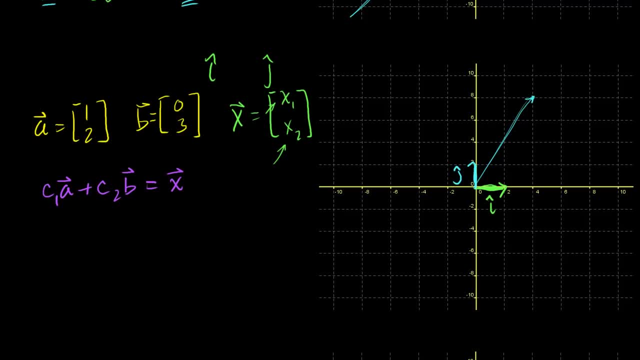 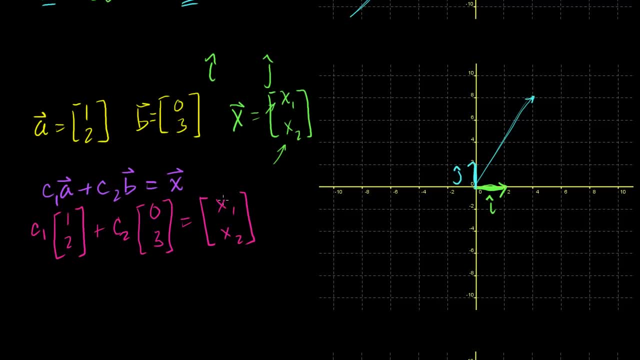 0, 3.. I should be able to be equal to my x1 and x2, where these are just arbitrary, So let's see if I can set that to be true. So if this is true, then the following must be true: 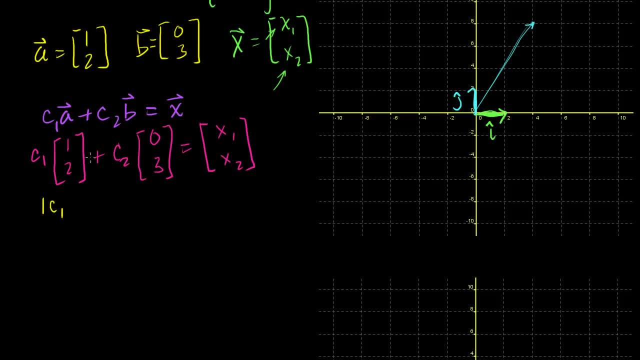 c1 times 1 plus 0 times c2 must be equal to x1.. We just get that from our definition of multiplying vectors, times scalars and adding vectors. And then we also know that 2 times c2, sorry, 2 times c1. 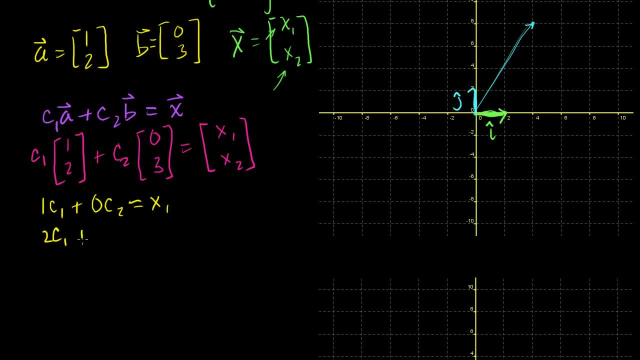 equals 1.. c1 times 2 plus c2 times 3, 3c2, should be equal to x2.. Now if I can show you that I can always find c1's and c2's, given any x1's and x2's, then I've proven that I can get to. 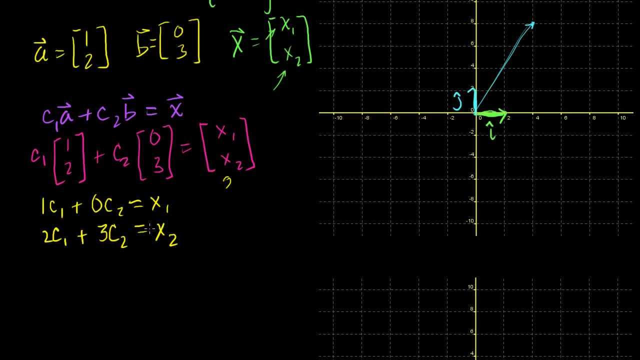 any point in R2, using just these two vectors. So let me see if I can do that. So this is just a system of two unknowns. This is just a 0, we can ignore it. So let's multiply this equation up here by minus 2. 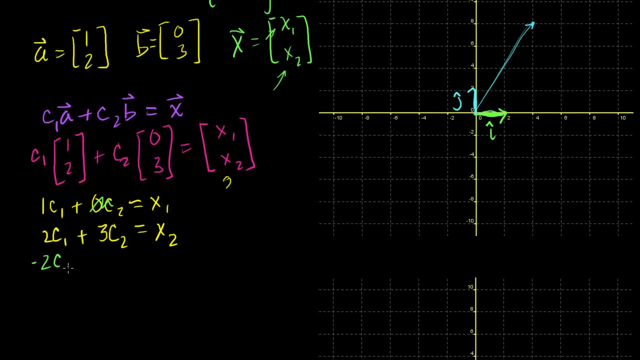 and put it here. So we get minus 2c1, I'm just multiplying this times minus 2, we get a 0 here plus 0 is equal to minus 2x1.. And then you add these two, you get 3c2, these cancel out. 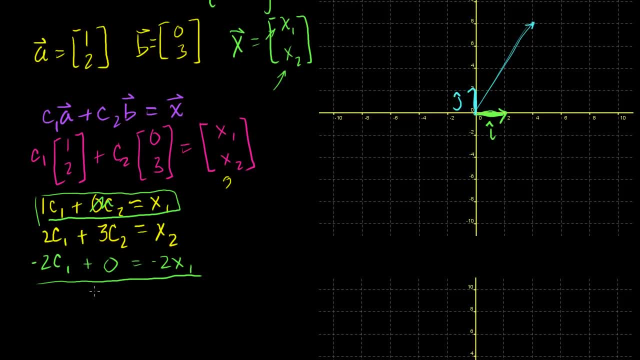 you get 3,. let me write in a different color. you get 3c2 is 0.. You get 3c2 is equal to x2 minus 2x1.. Or divide both sides by 3, you get c2 is equal to 1 third x2. 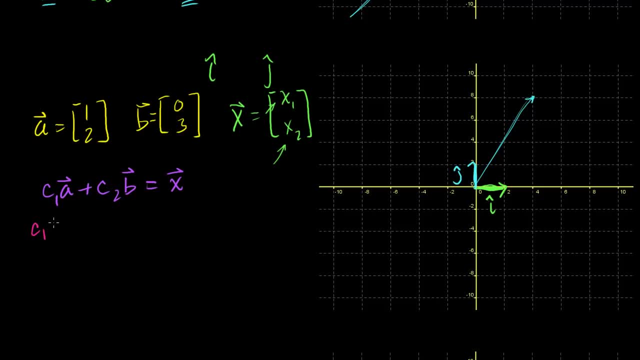 being represented in their kind of column form. So we have c1 times this vector plus c2 times the b vector. 0, 3 should be able to be equal My x2.. This vector should be able to be equal to my x1 and x2,. 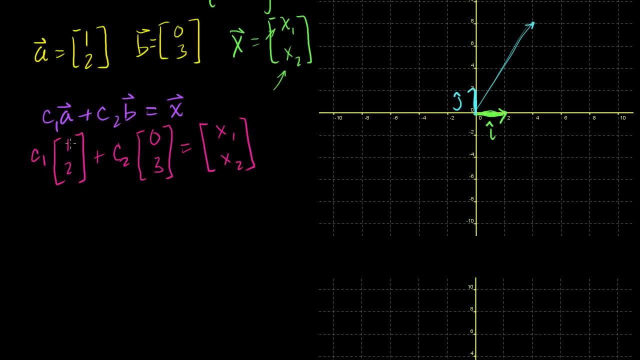 where these are just arbitrary. So let's see if I can set that to be true. So if this is true, then the following must be true: c1 times 1 plus 0 times c2 must be equal to x1.. We just get that from our definition of multiplying. 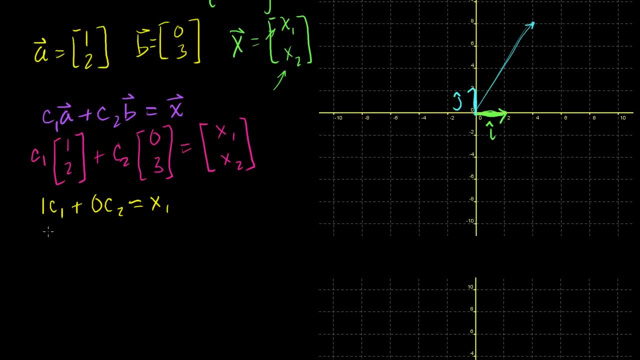 vectors, times, scalars and adding vectors. And then we also know that 2 times c2, sorry, 2 times c1 times 2 plus c2 times 3, 3c2, should be equal to x2.. Now if I can show you that I can always find c1's and c2's, 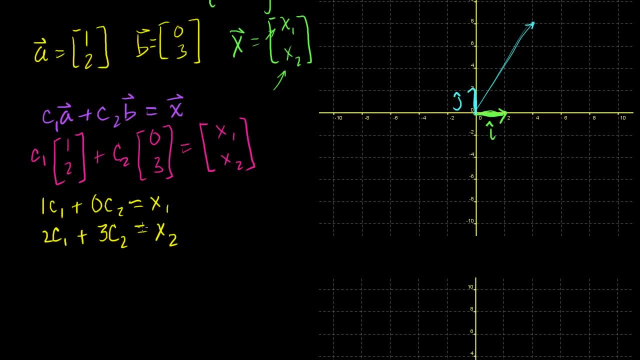 given any x1's and x2's, then I've proven that I can get to any point in R2 using just these two vectors. So let me see if I can do that. So this is just a system of two unknowns. 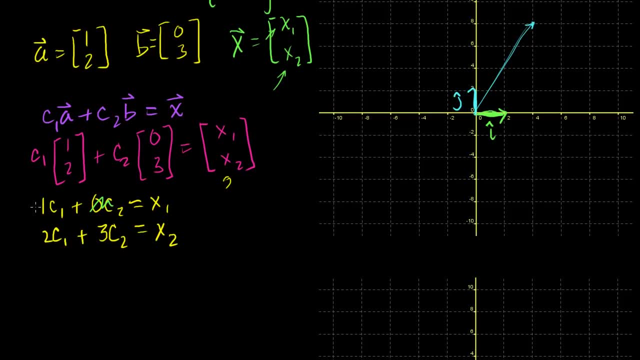 This is just a 0.. We can ignore it. So let's multiply this equation up here by minus 2 and put it here, so we get minus 2c1.. I'm just multiplying this times minus 2.. We get a 0 here. 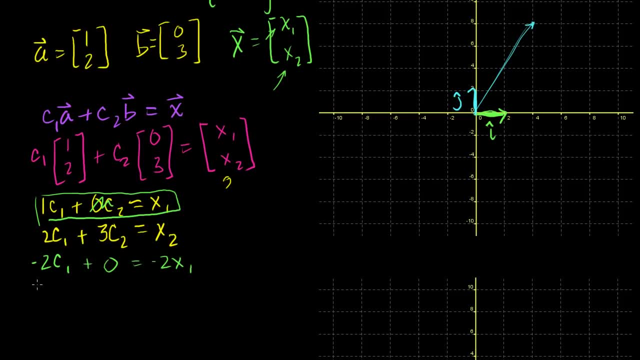 Plus 0 is equal to minus 2x1.. And then you add these two, You get 3c2.. These cancel out, You get 3.. Let me write it in a different color: You get 3c2.. 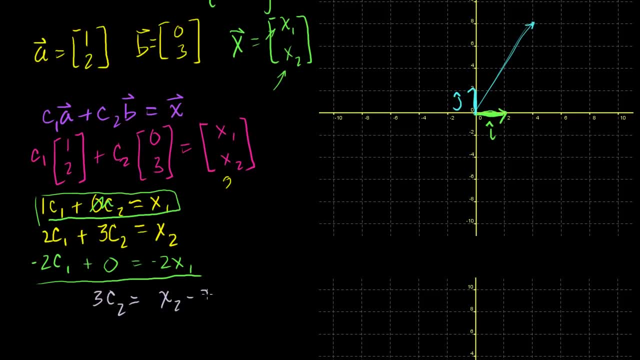 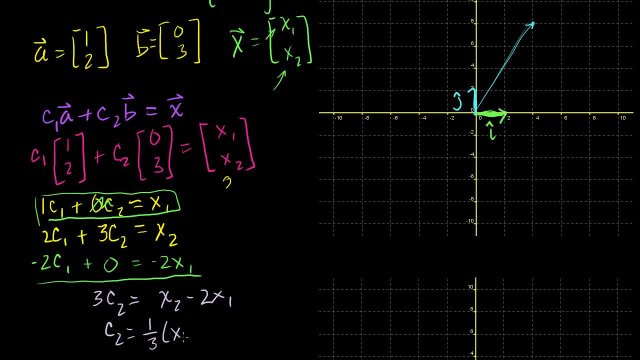 You get: c2 is equal to 1 third x2 minus x1.. Now we'd have to go substitute back in for c1. Well, we have this first equation right here, that c1. This first equation just says c1 plus 0 is equal to x1. 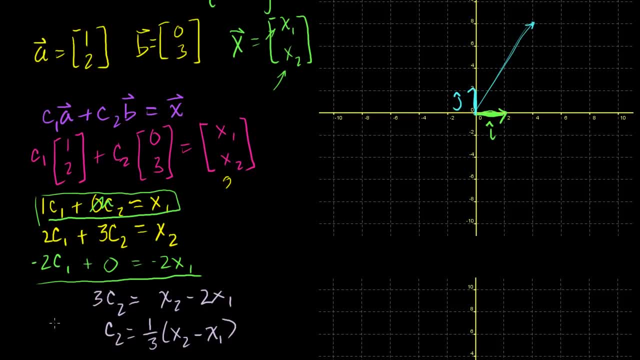 minus x1. Now we'd have to go substitute back in for c1. Well, we have this first equation right here, that c1, this first equation just says c1 plus 0 is equal to x1. So c1 is equal to x1. 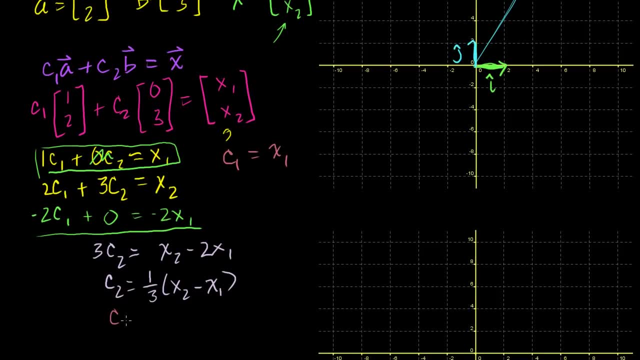 So that one just gets us there. So c1 is equal to x1.. So you give me any point in R2, these are just two real numbers and I can just perform this operation and I'll tell you what weights to apply to a and b to get to that point. 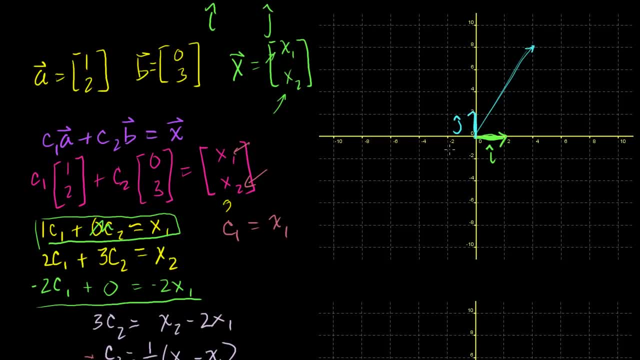 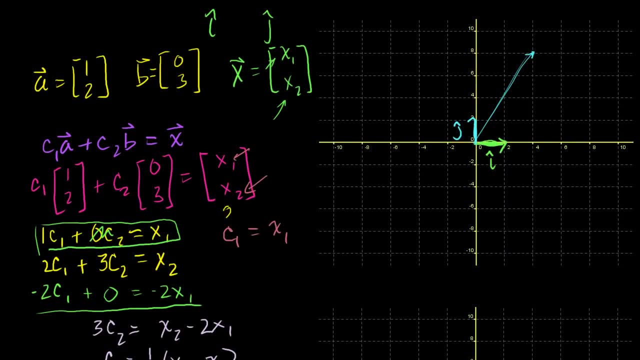 If you say, OK, what combination of a and b can get me to the point? let's say I want to get to the point, let me go back up here. well, it's way up there. Let's say I'm looking to get to the point 2, 2.. 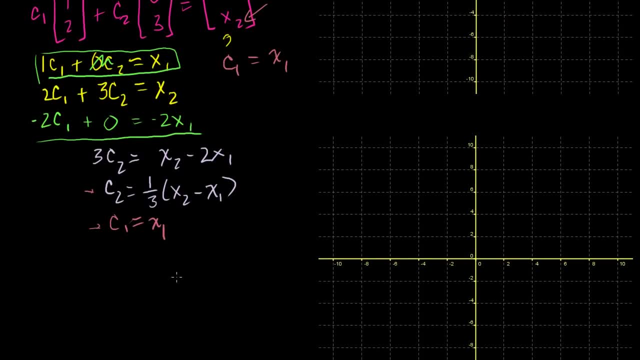 So x1 is 2.. Let me write it down here. Say- I'm trying to get to the point- the vector 2, 2.. What combinations of a and b can be there? Well, I know that c1 is equal to x1, so that's equal to 2.. 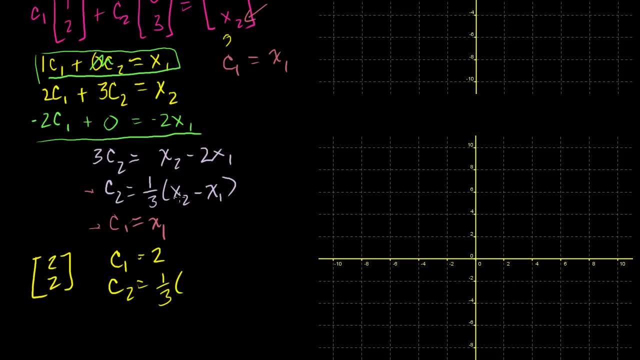 And c2 is equal to 1 third times 2 minus 2.. So 2 minus 2 is 0. So c2 is equal to 0.. So if I want to just get to the point 2, 2, I just have to go. 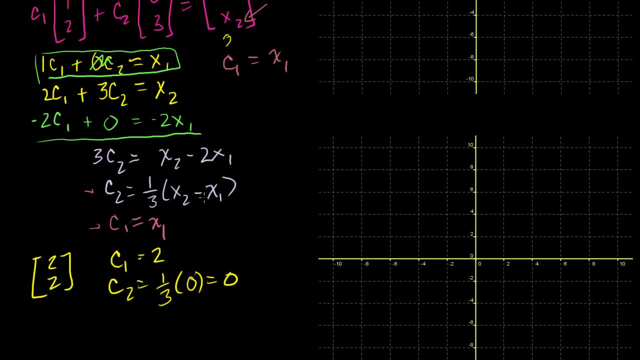 ahead and just multiply. Oh, I just realized this was looking suspicious. I made a slight error here and this was good that I actually tried it out with real numbers Over here when I had: 3c2 is equal to x2 minus 2x1, I got. 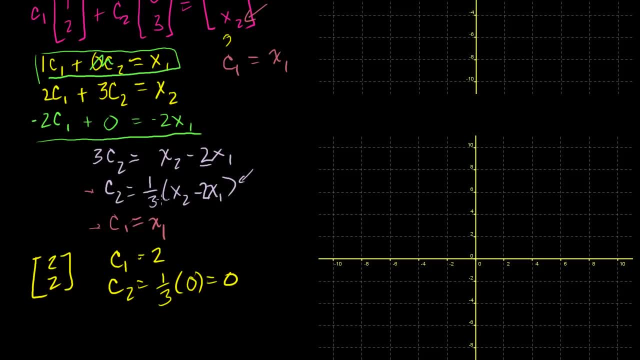 rid of this 2 over here. There's a 2 over here. I divide both sides by 3.. I get 1 third times x2 minus 2x1.. And that's why I was like, hey, this is looking strange. 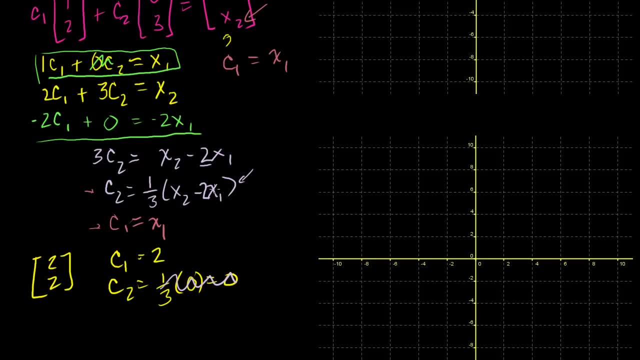 So I had to take a moment of pause. So let's go to my corrected definition of c2.. c2 is equal to 1 third 2 times x2.. So 2 minus 2 times x1.. So minus 2 times 2.. 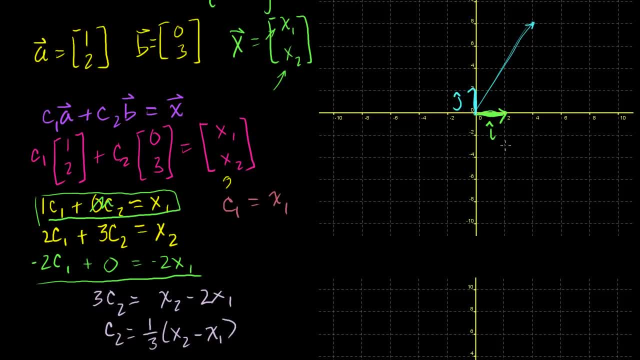 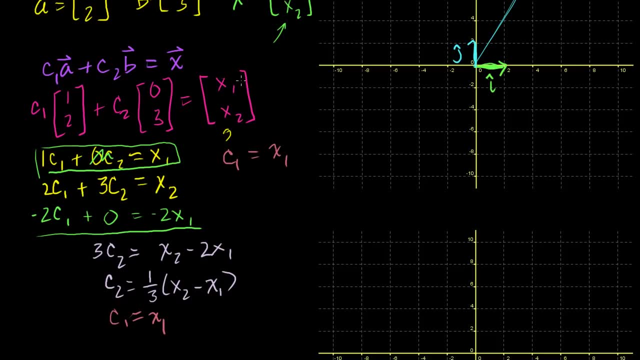 So c1 is equal to x1.. So that one just gets us there. So c1 is equal to x1.. So you give me any point in r2.. These are just two real numbers And I can just perform this operation. 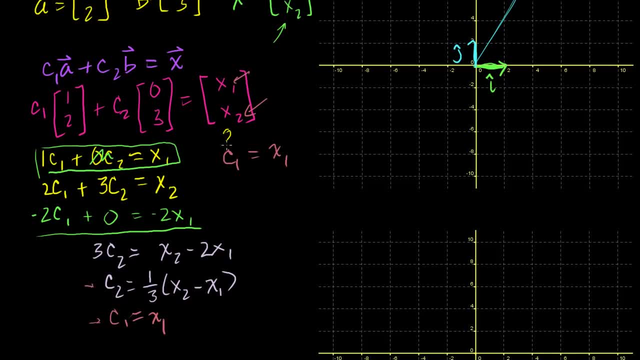 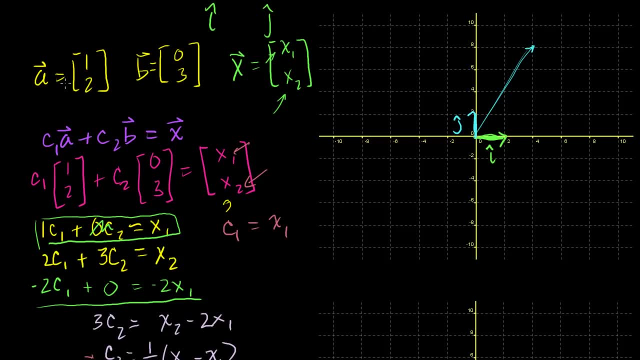 And I'll tell you what weights to apply to a and b to get to that point. If you say OK, what combination of a and b can get me to the point? Let's say I want to get to the point. Let me go back up here. 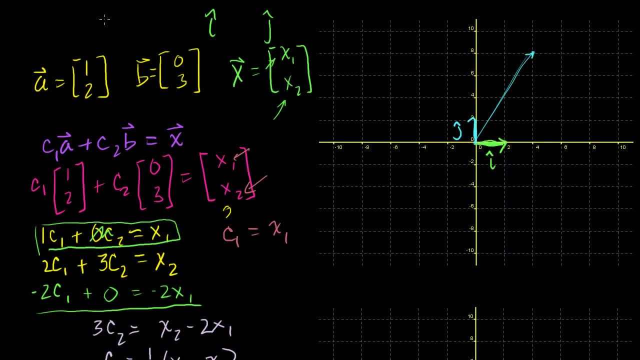 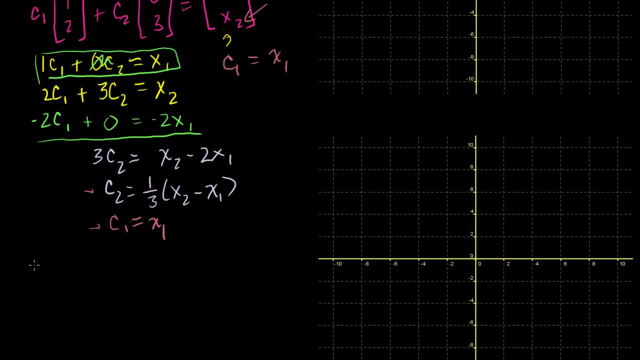 Well, it's way up there. Let's say I'm looking to get to the point 2, 2.. So x1 is 2.. Let me write it down here, Say I'm trying to get to the point the vector 2, 2.. 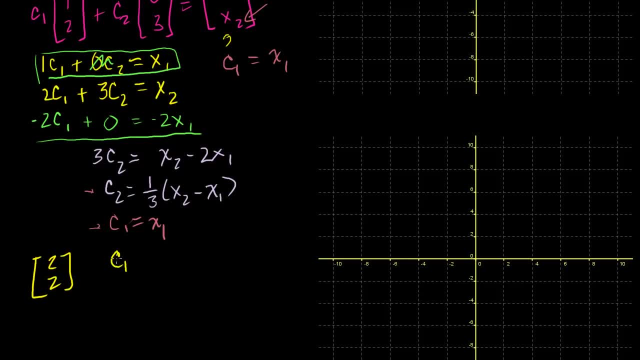 What combinations of a and b can be there? Well, I know that c1 is equal to x1.. So that's equal to 2.. And c2 is equal to 1, third times 2 minus 2.. So 2 minus 2 is 0. 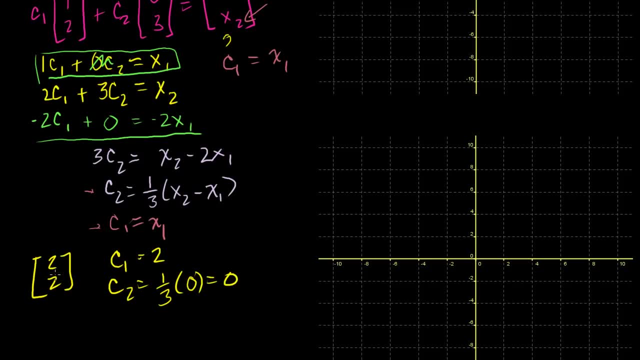 So c2 is equal to 0.. So if I want to just get to the point 2,, 2,, I just multiply. Oh, I just realized This was looking suspicious. I made a slight error here And this was good that I actually tried it out with. 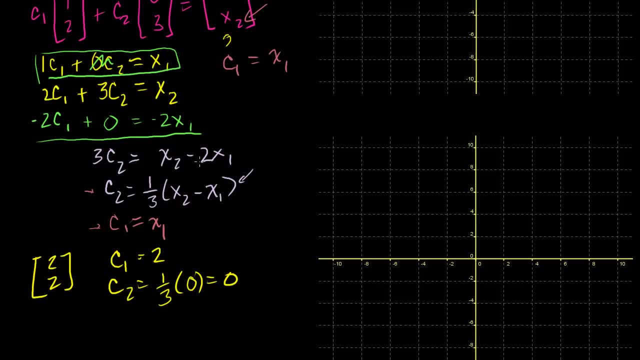 real numbers Over here. when I had 3c2 is equal to x2 minus 2x1, I got rid of this 2 over here. There's a 2 over here. I divide both sides by 3. I get 1 third times x2 minus 2x1.. 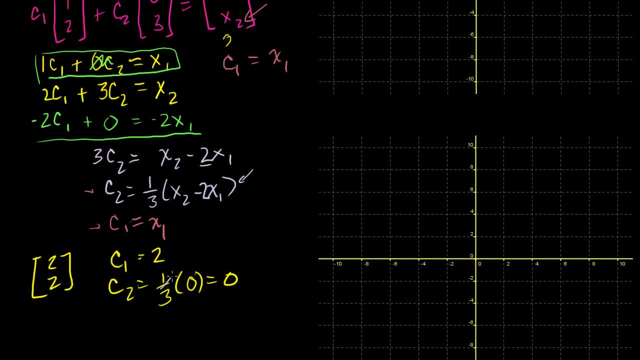 And that's why I was like, hey, this is looking strange, So I had to take a moment of pause. So let's go to my corrected definition of c2.. c2 is equal to 1 third, 2 times x2.. 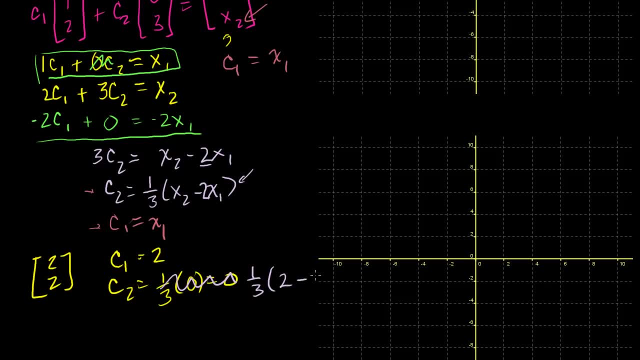 So 2 minus 2 times x1.. So minus 2 times 2.. So it's equal to 1 third times 2 minus 4, which is equal to minus 2, so it's equal to minus 2 thirds. 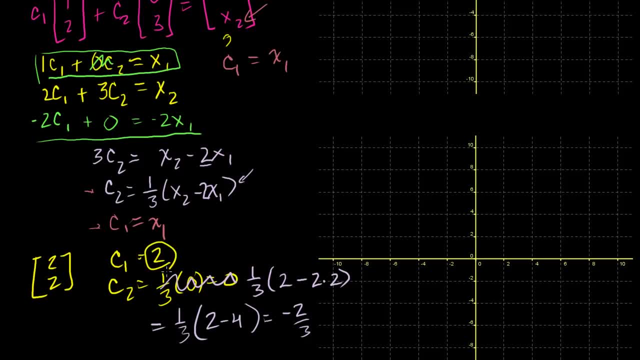 So if I multiply 2,, 2 times my vector a, minus 2 thirds times my vector b, I will get To the third, The vector 2, 2.. And you can verify it for yourself: 2 times my vector a: 1, 2, minus 2 thirds times my vector.